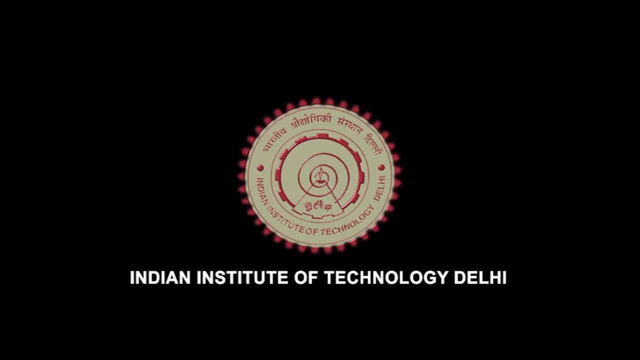 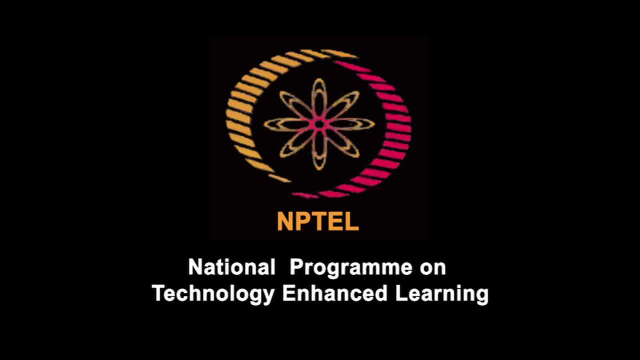 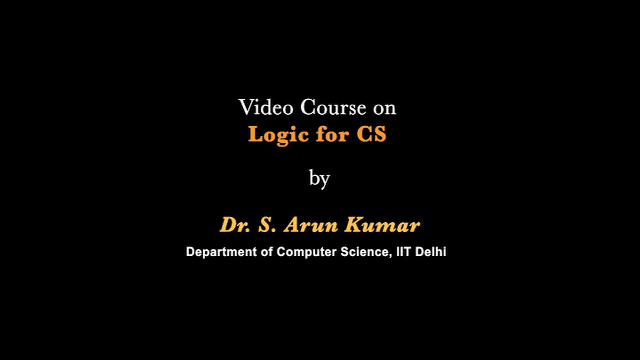 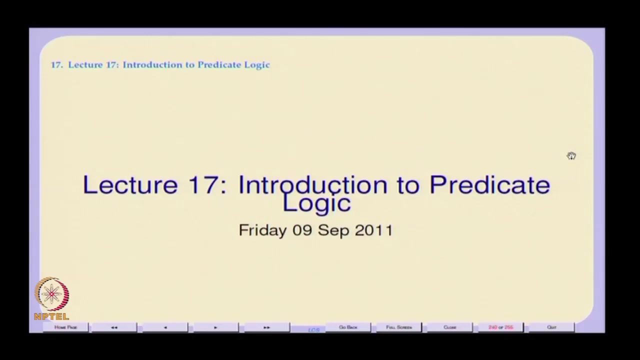 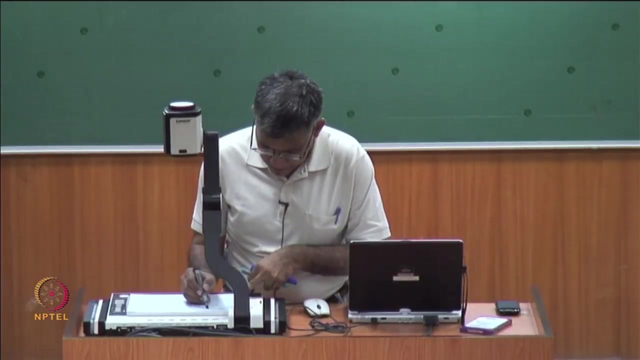 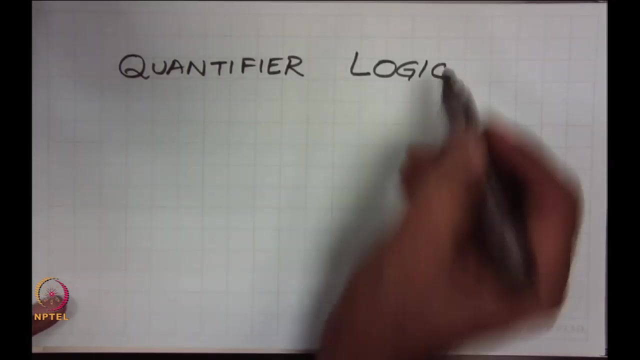 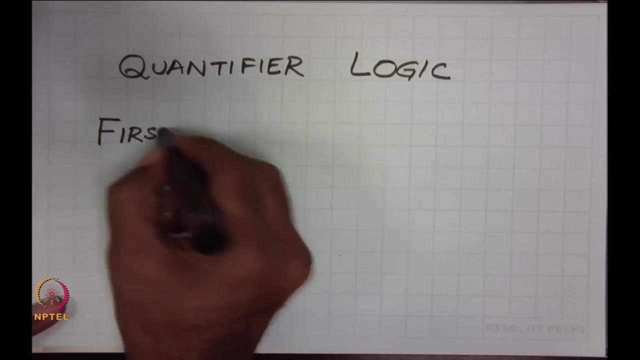 So we are going to introduce predicate logic. Predicate logic is also called- sometimes it is called quantifier logic. It is also sometimes- and the version we are going to study is specifically is called first order logic, And the question of what exactly first order means is something that I will discuss in the next. 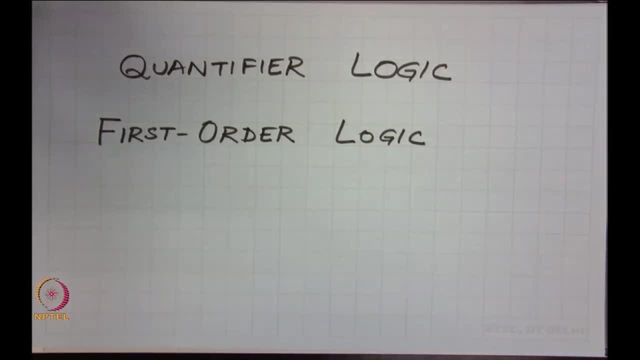 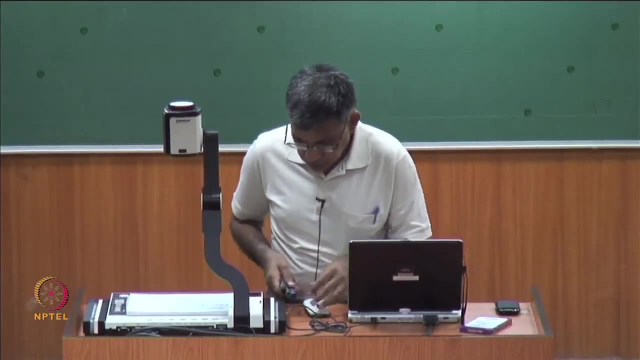 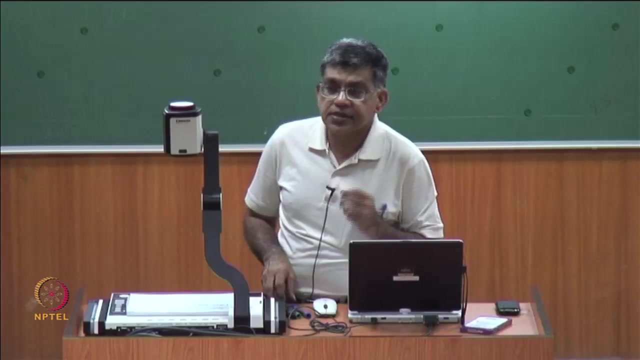 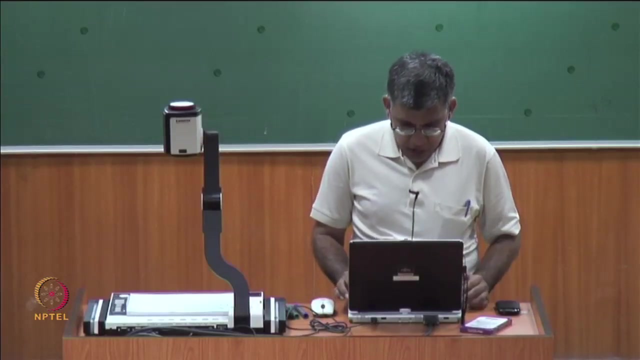 lecture I will talk about later, after we have defined the syntax, maybe. So let us start with predicate logic or quantifier logic. So the important thing to realize is that there is something about, or maybe I will come to that as we proceed. So the most famous valid argument. 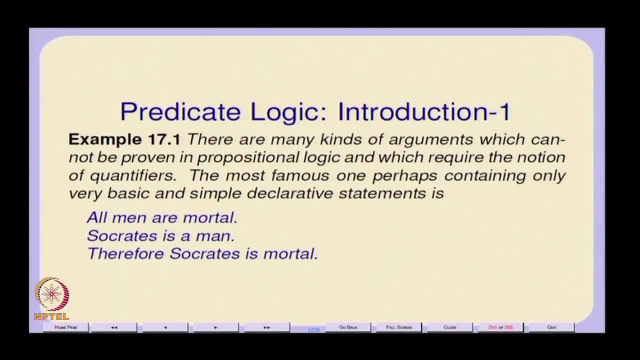 since the time of Aristotle, which introduces the subject- I mean might as well do this- Is this famous thing that all men are mortal. Socrates is a man, therefore Socrates is mortal, I mean. So the interesting thing about this argument is that all the sentences are very 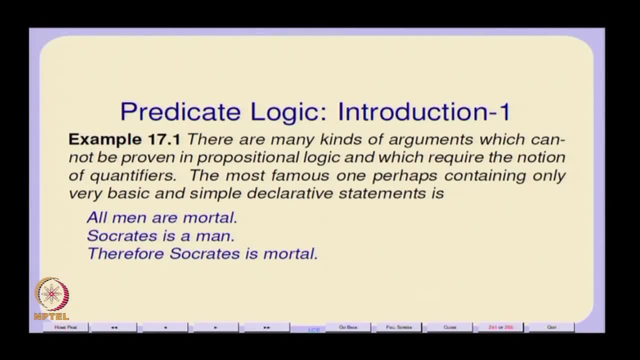 simple sentences. There are no propositional connectives. So there is, and yet it is sort of a valid argument, and what we would like to know is exactly: therefore, what is lack? it is not provable in propositional logic, Since all of them. 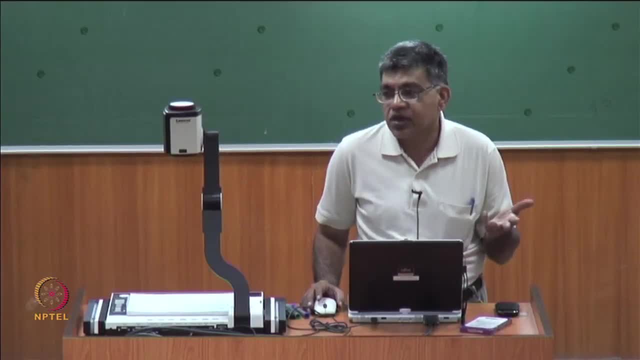 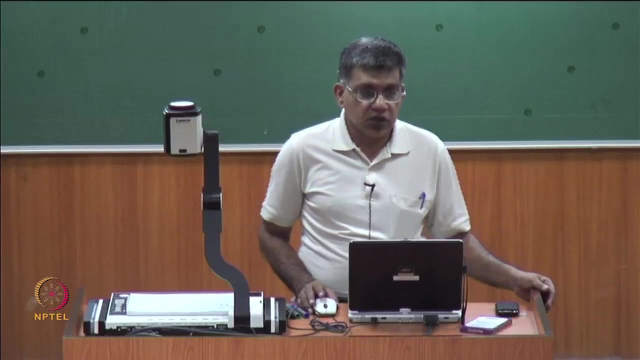 are simple sentences. you will give all of them separate propositional symbols. I mean, they cannot be broken up and they are not compound propositions, they are all simple propositions. So essentially, you will never be able to prove the validity of this argument from propositional. 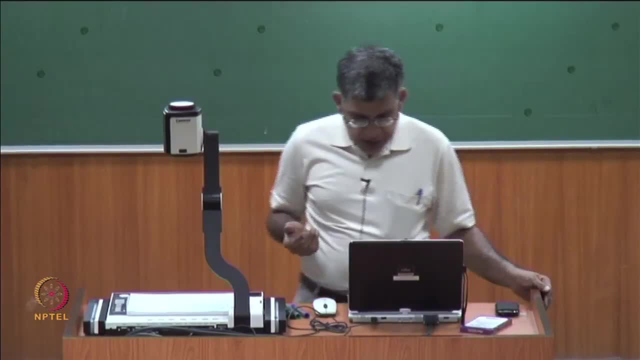 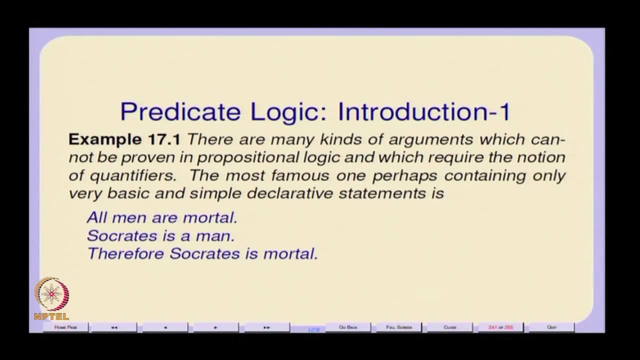 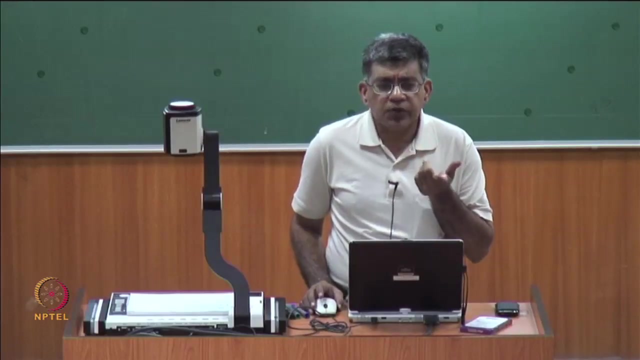 logic. So there are other similar things, but what we should do is instructive: to just look at this argument and see, therefore, what is actually lacking in propositional logic. 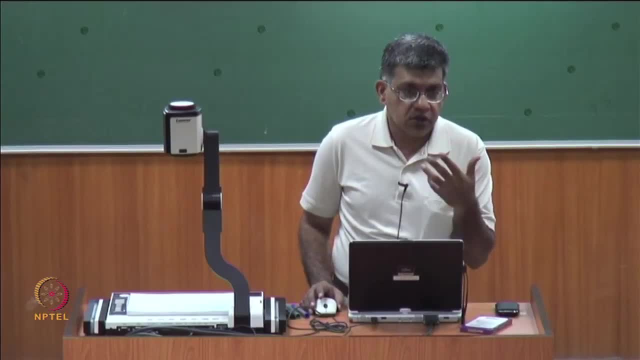 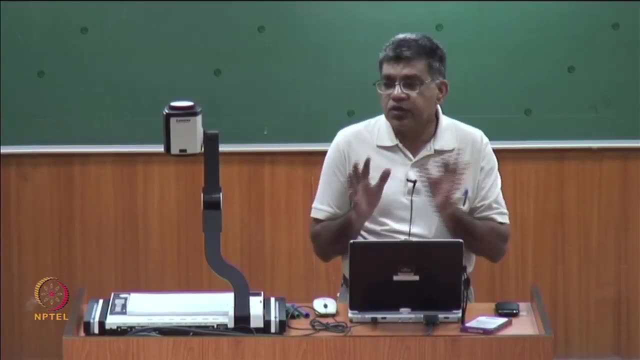 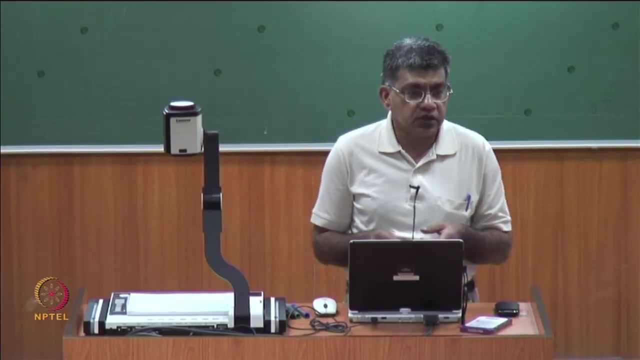 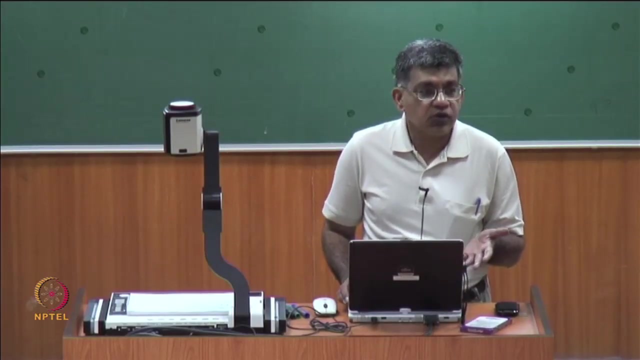 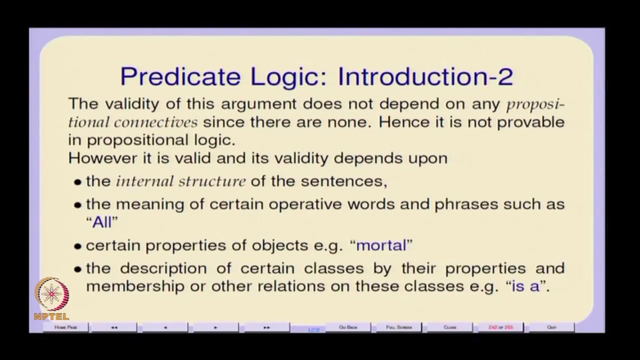 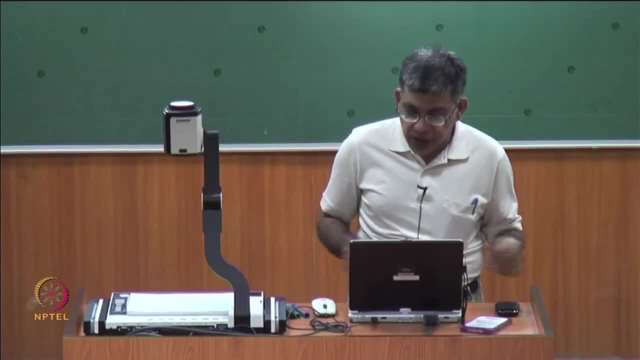 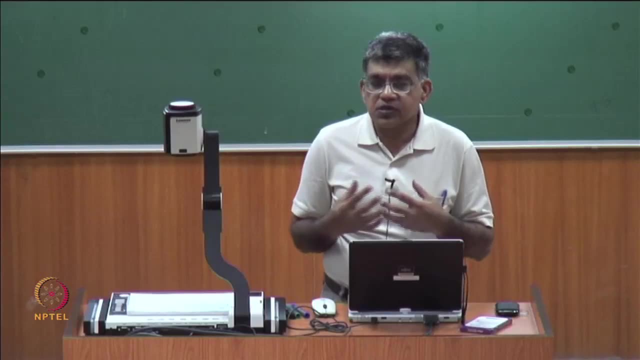 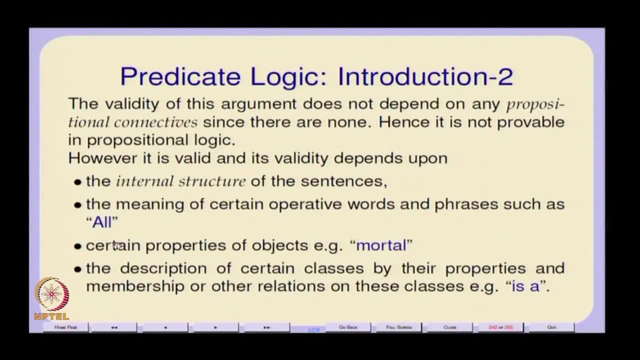 There are certain key words, like all and some, and there are certain properties which are essentially like. they are in a linguistic sense, they are like adjectives, they are not prepositions or conjunctions. So there are properties of certain objects, like mortal, for example, and then there is a description of essentially 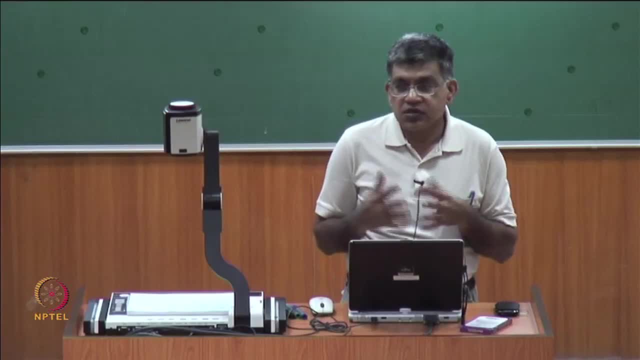 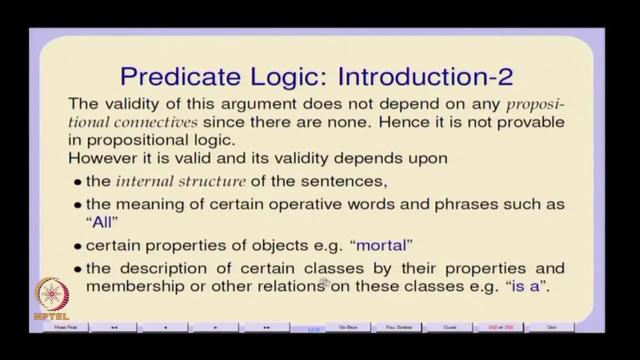 classes of objects, that is, which is not there in the propositional case. So which means that so the, and then when you are talking about classes, you are essentially talking about membership in classes and you are talking about, sometimes, relationships between different classes. So if you look at so predicate, logic essentially means that there 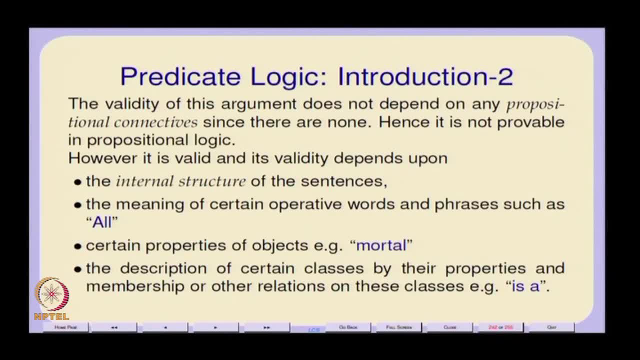 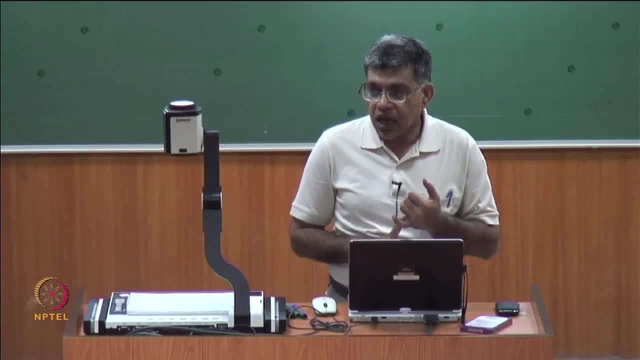 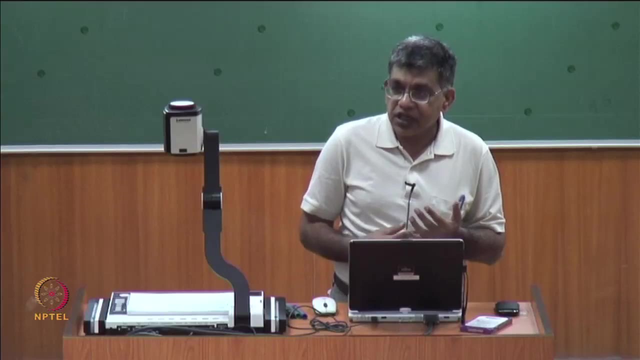 is something in the internal structure which somehow has to bring into, take into account classes, relationships between classes of objects and not I mean. So any argument that goes beyond singular objects or individual objects requires a different kind of treatment. So, linguistically, there is this question of looking at adjectives which are like properties. 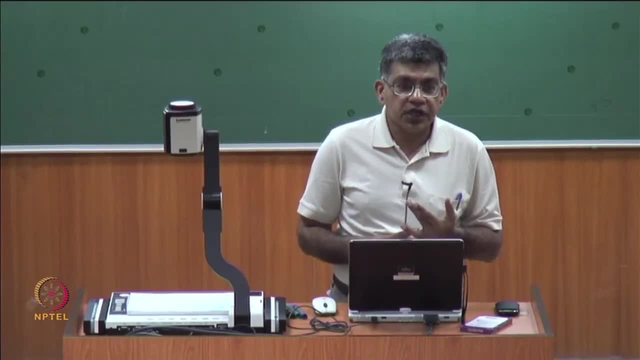 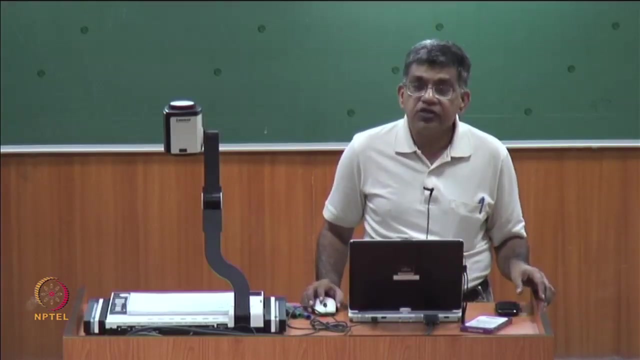 relationships, So classes of objects, the relationship of individuals to classes, essentially membership in classes, and these kinds of things somehow come out from the internal structure of these sentences and till you have actually formalize them, it is unlikely that you are ever going to be able to prove that such a simple argument, which is sort of obviously valid, should also. 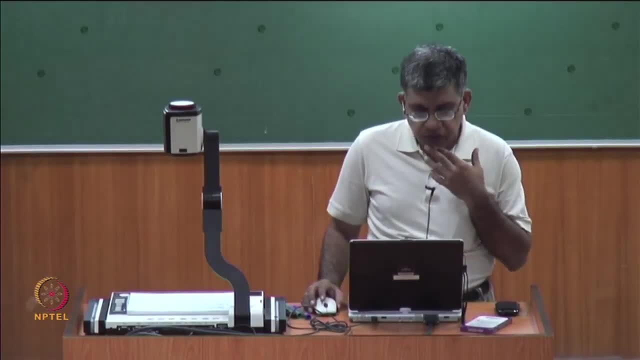 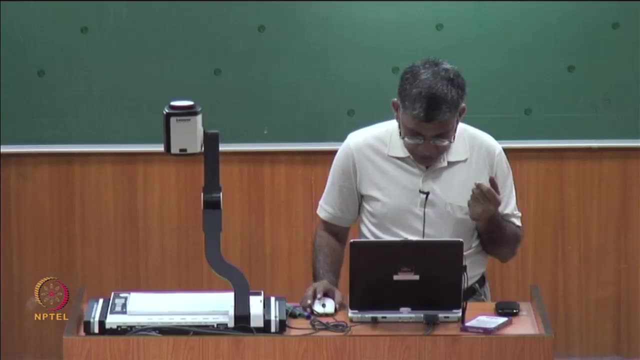 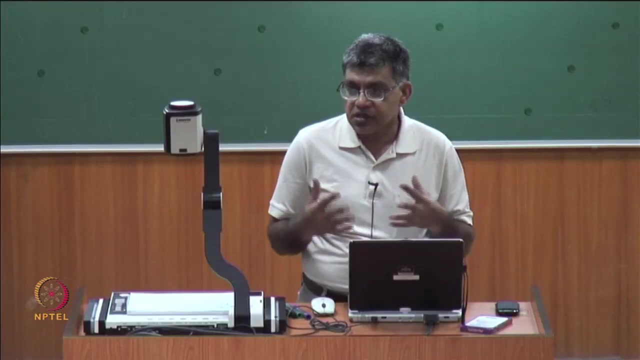 be is also valid. So there are other kinds of arguments which are- And it is categorical in that sense, supposing you had, all cats are mammals, some mammals. 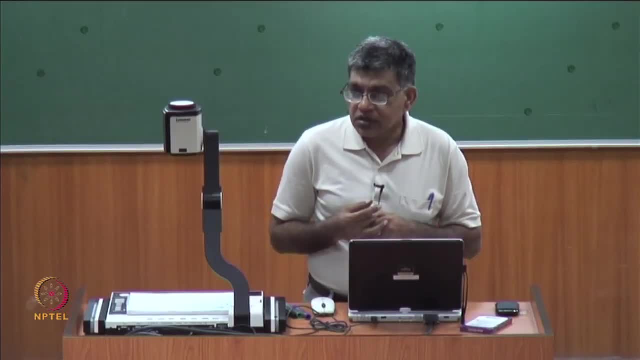 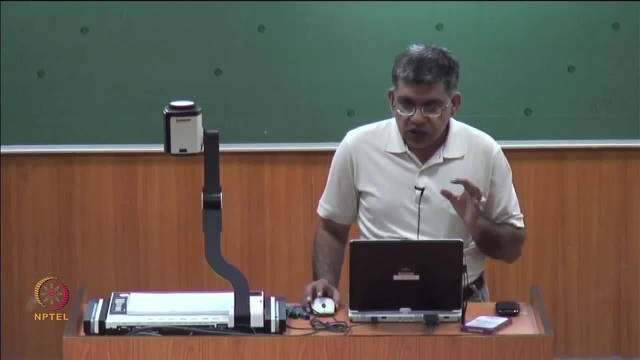 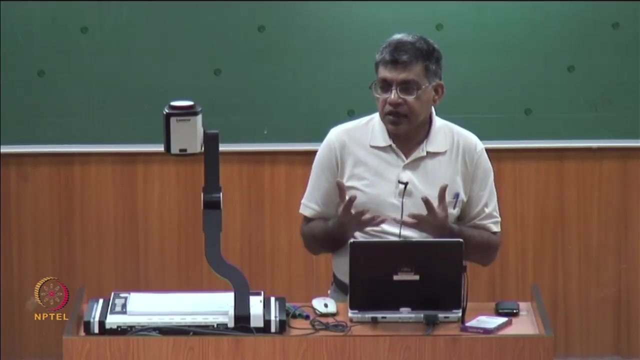 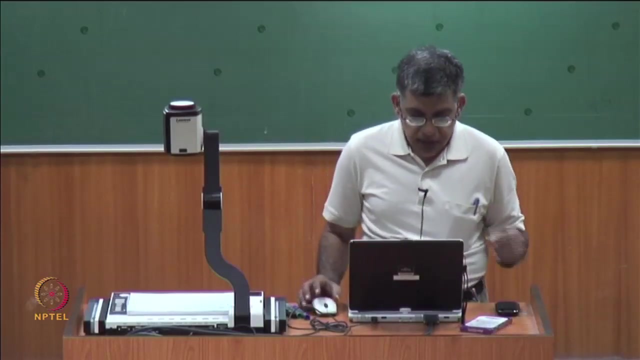 do not have vertebrae, some cats do not have vertebrae, therefore, some mammals do not have vertebrae, For example. so there are some specializations of all and some and which are, which make these categorical propositions. so you need to look deeper into their structure so that so, and 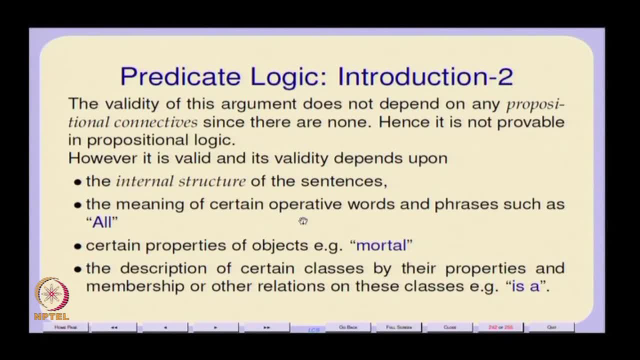 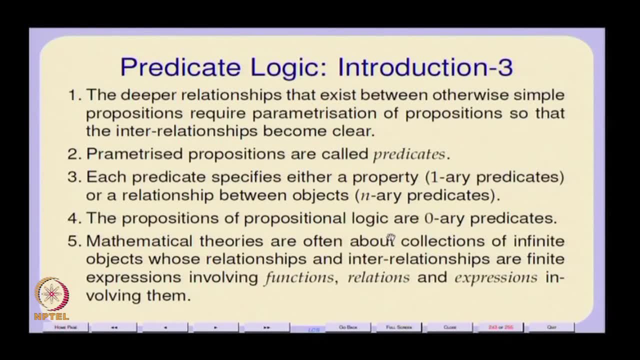 mathematically speaking, of course. actually it is the most obvious thing to do is to actually parameterize propositions. So you sort of parameterize the propositions, so what we will have are parameterized propositions, and these parameterized propositions are called predicates, from which the logic gets its name. 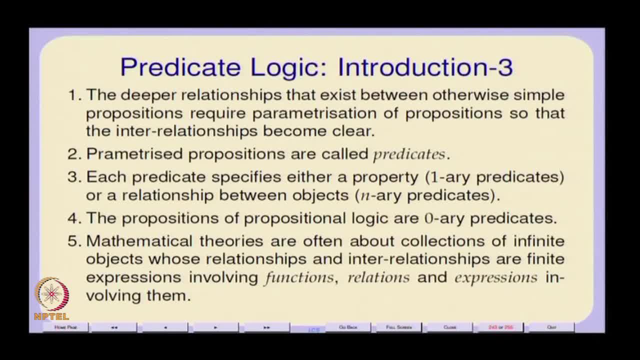 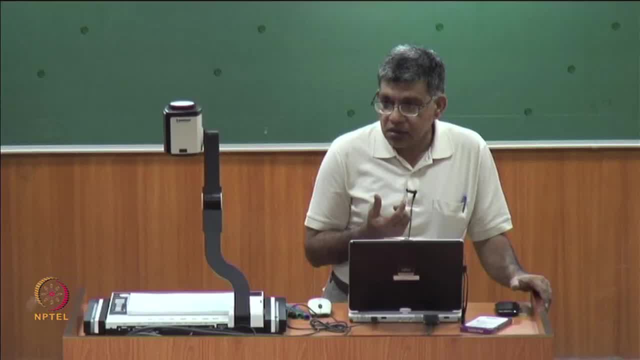 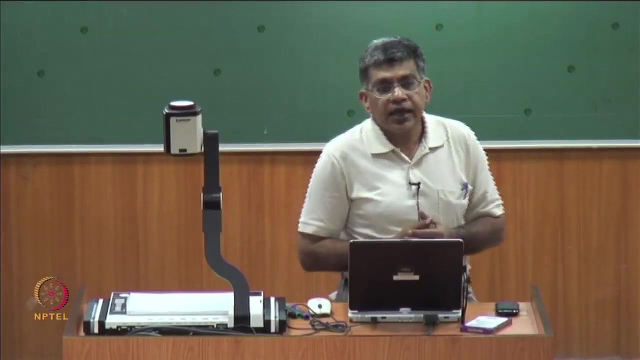 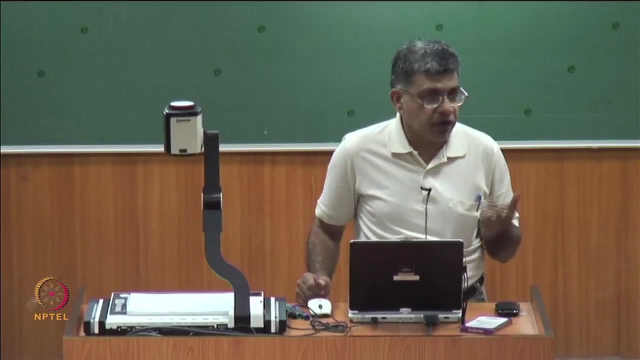 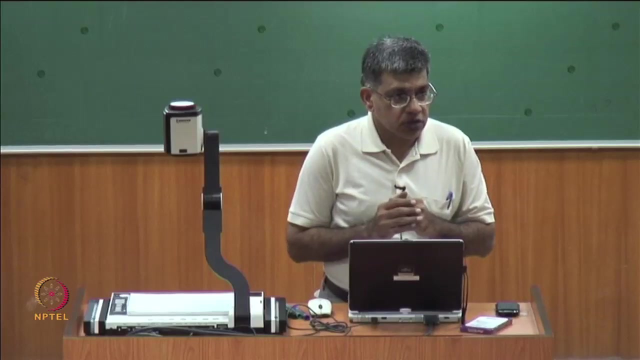 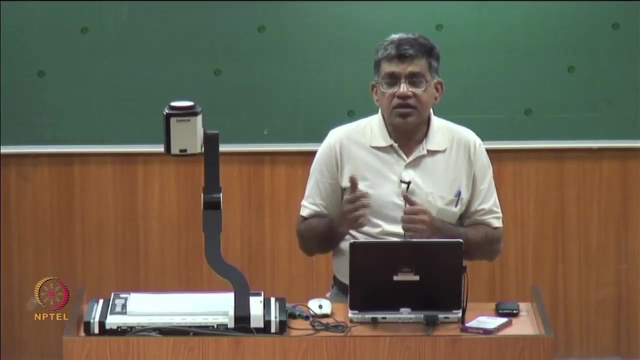 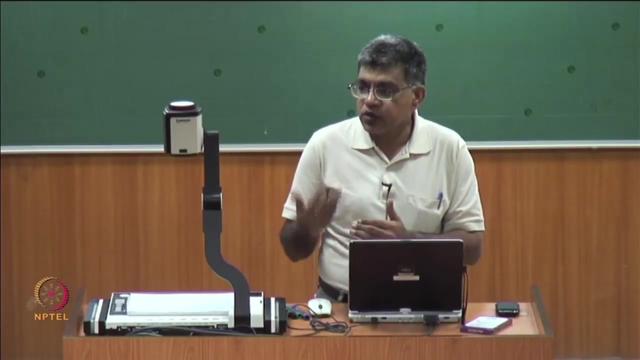 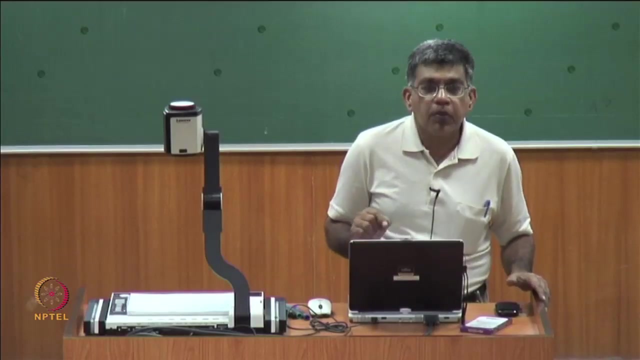 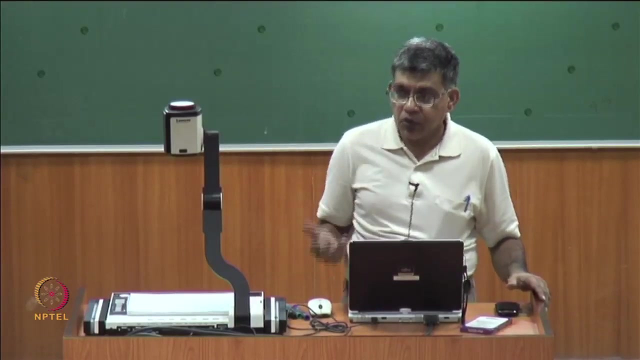 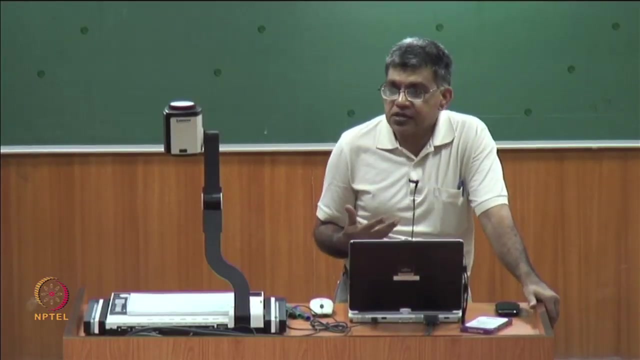 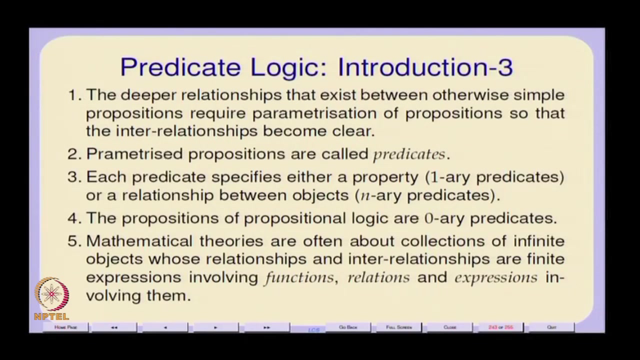 so a proposition, by whatever we have so far seen, is something, is a declarative statement. So when you think of parameterized propositions, you can also think of them as like going from propositions which are like constants to propositional functions which are propositions. 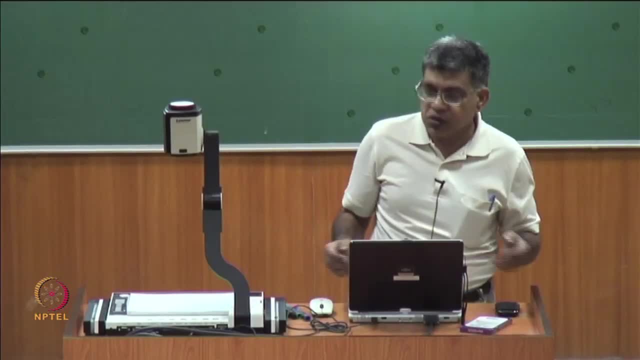 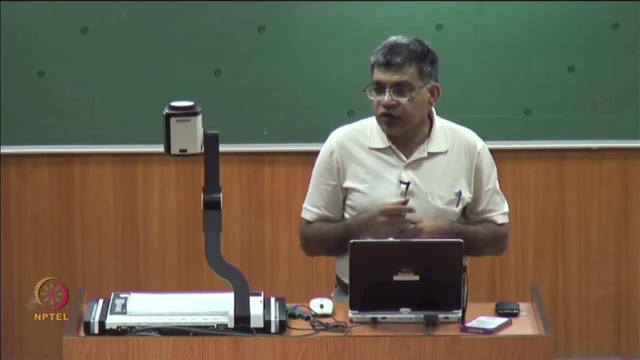 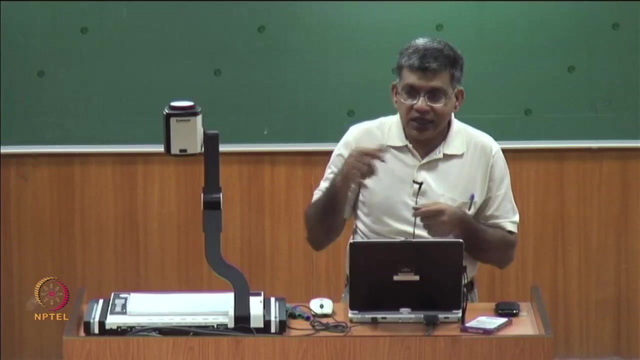 of some variables. So predicates can also be thought of as propositional functions. so where the placeholders? there might be many different placeholders and they establish a certain structure. That is why truth or falsehood cannot be determined till values are actually substituted in the various places. 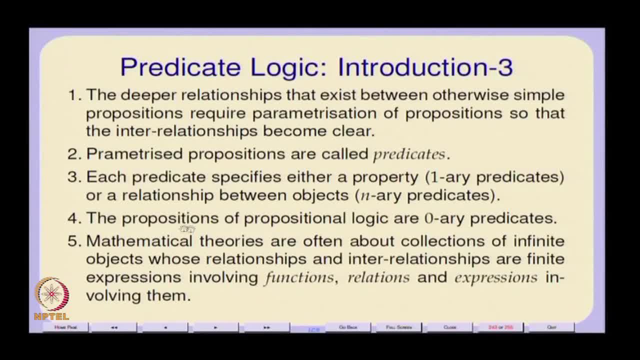 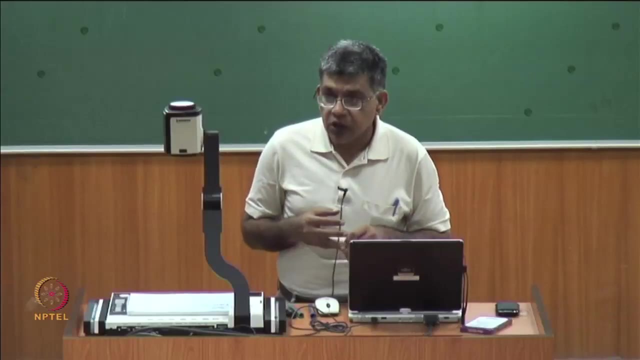 So the other way to look at things is that the propositions of propositional logic are 0 Array predicates, and important thing here now is that we have this. So essentially, our primary purpose, besides a linguistic, besides a pure definition, So decides a purely linguistic for into logic, is also to that is, that of describing. 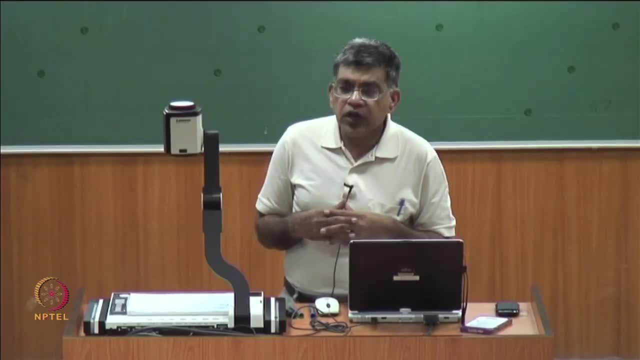 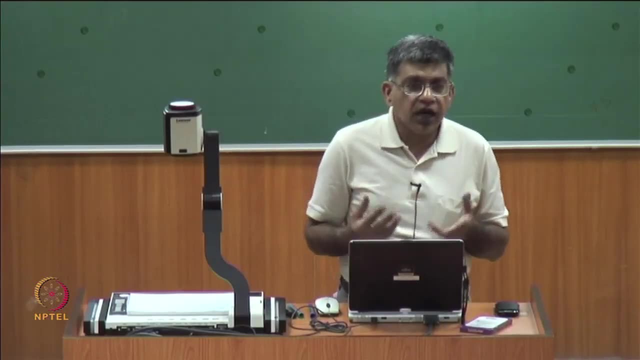 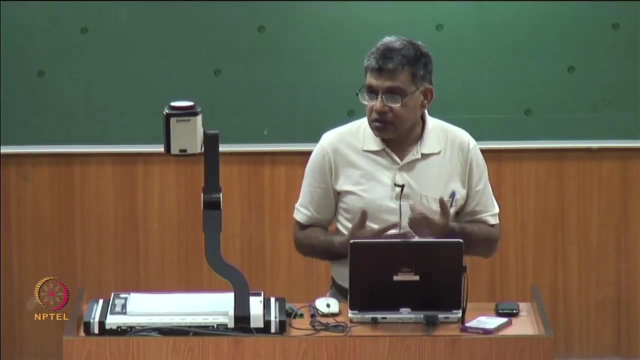 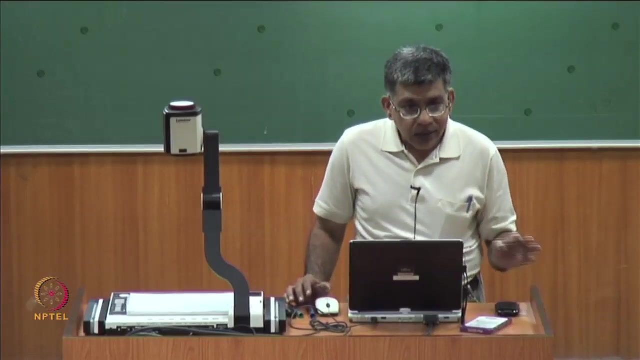 mathematical theories right. So when you look at any mathematical theory, group theory for example, then what you have there is a high prevalence of functions and relations and expressions involving functions and relations. So, which means that- and they are about, very often they are about these: 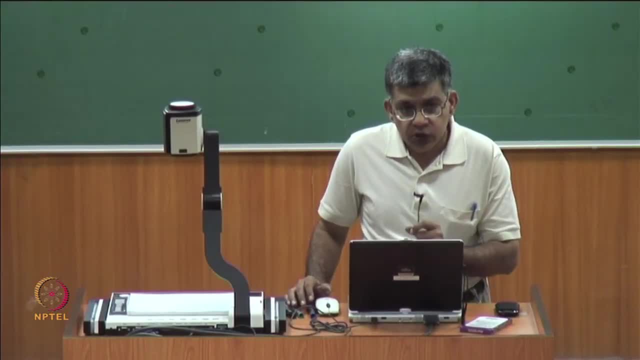 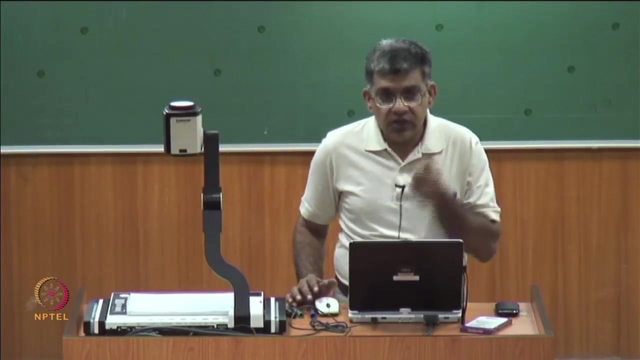 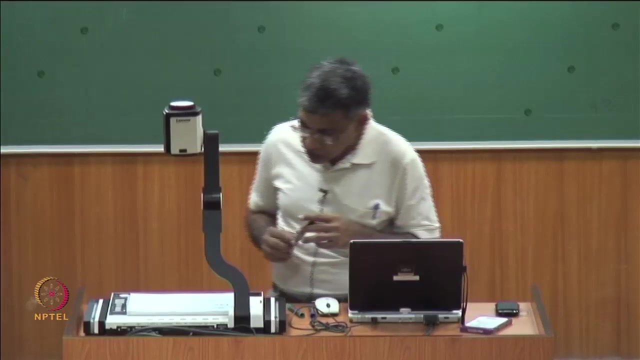 functions and relations often are used to describe infinitary objects or infinite classes in some finitary representation, right. So bringing down the infinite to some finite expressibility is a proper exercise in mathematics, right, and that is, that is something that we have to take in to account and by and large, So by and large, whatever reasoning we do in this, 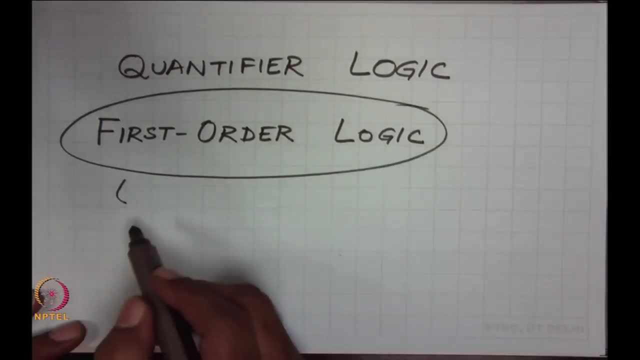 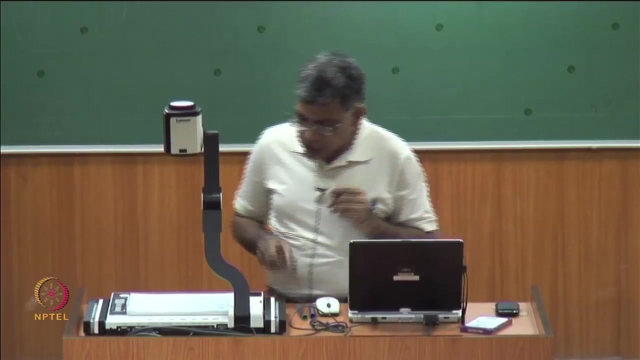 first order logic is more or less applicable to most mathematical theories. there is a subtle instance, there is a subtlety about the logic being first order and what that actually means. So what we will do is let us look at, let us think of propositional logic as essentially 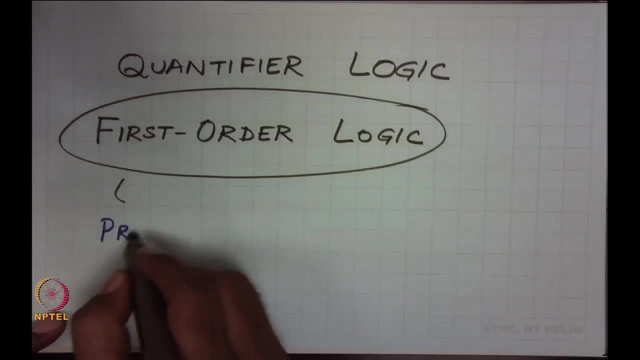 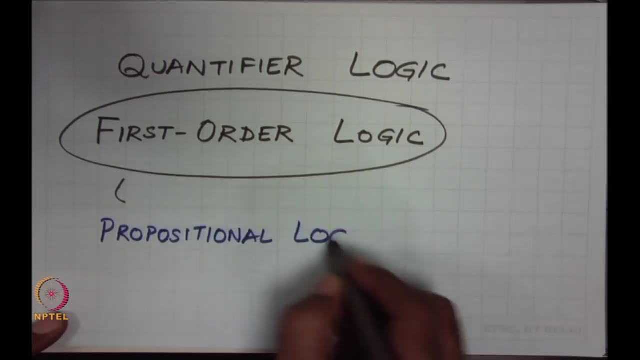 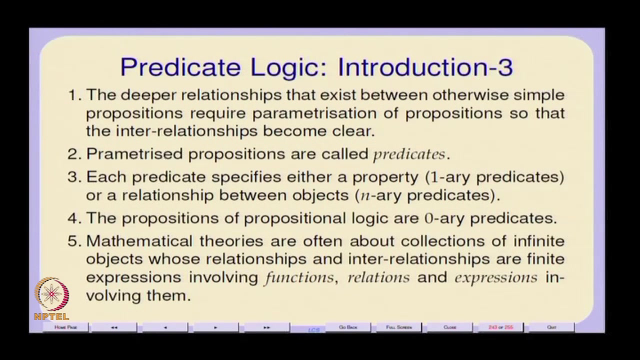 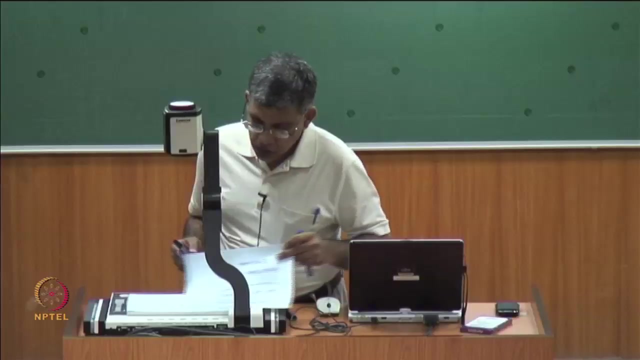 being zeroth order. So we will say that propositional logic is essentially zeroth order. So when we talk about predicates or first order logic, then what we are talking about is a class of individuals. So usually we are talking about a mathematical theory which 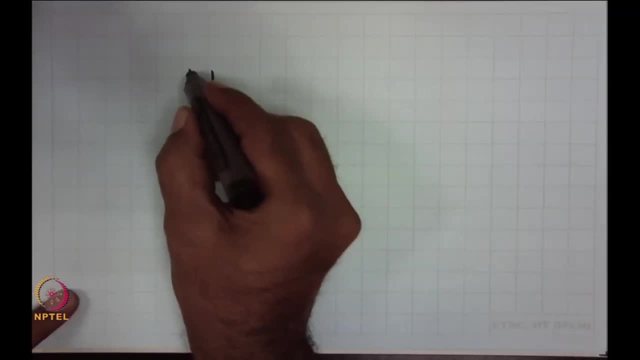 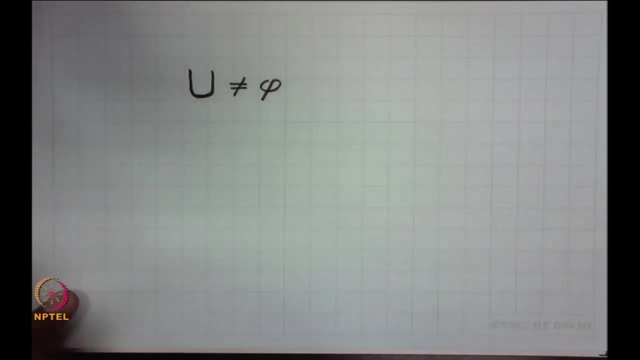 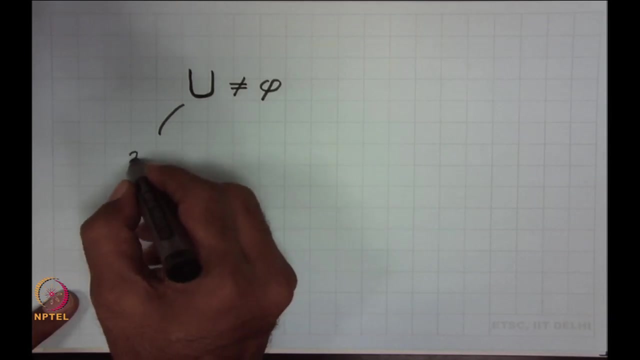 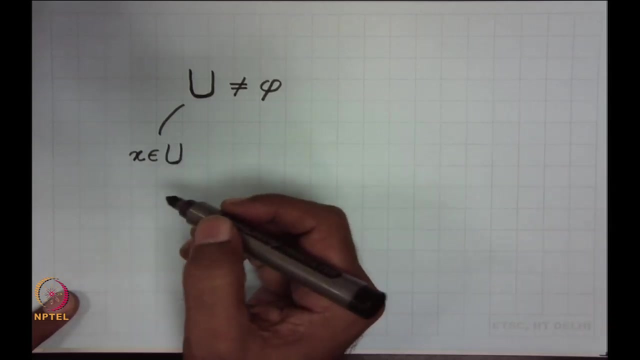 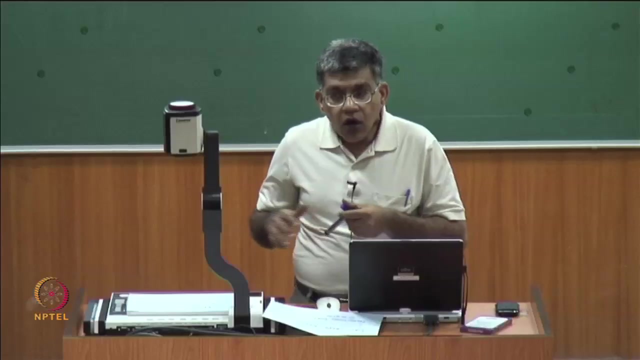 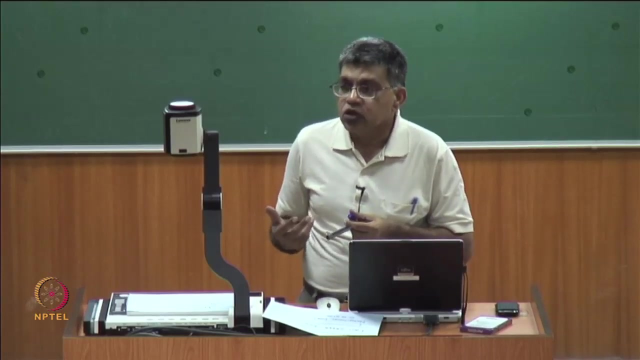 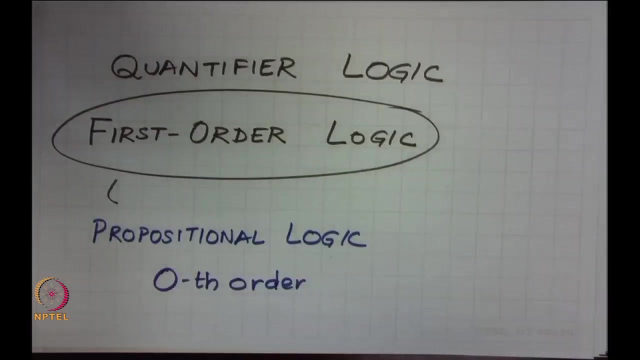 has some universal set, and this universal set is non-existent And what we are looking at are properties of, let us say, elements of this universal set. It is possible to look at properties of subsets of this universal set. So what makes a logic first order is the fact that you are not interested in properties. 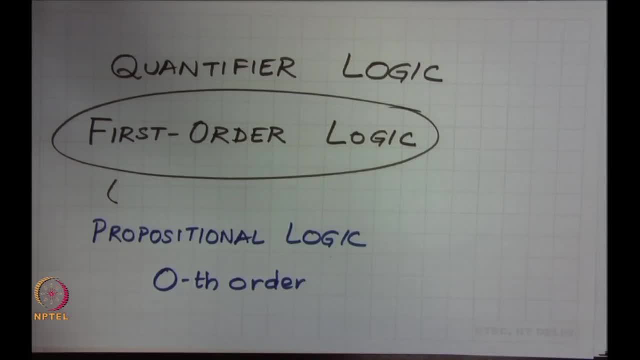 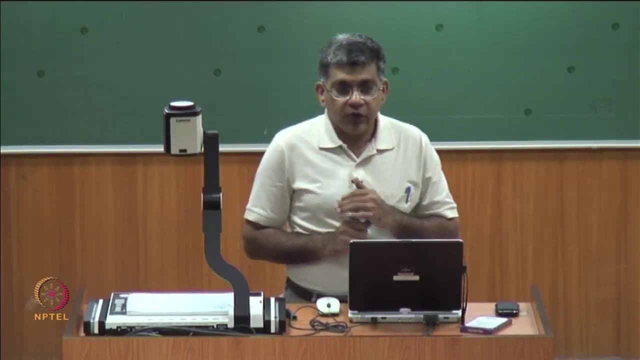 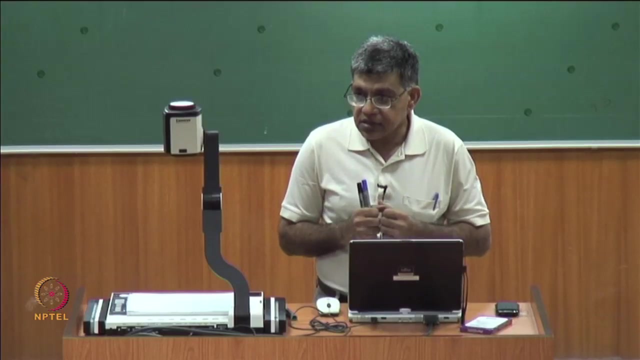 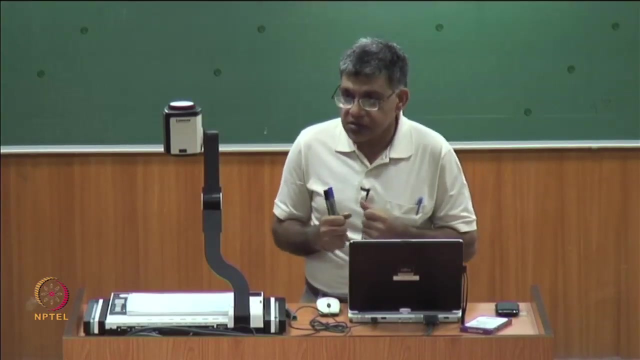 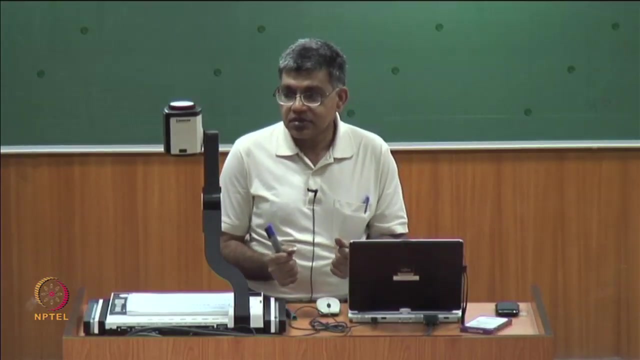 of subsets. You are interested only in properties of individuals. So you are looking at, you are looking at fairly general properties about individuals only in that set and you might be able to class various, characterize various subsets of this universal set by describing properties of individuals in some parameterized. 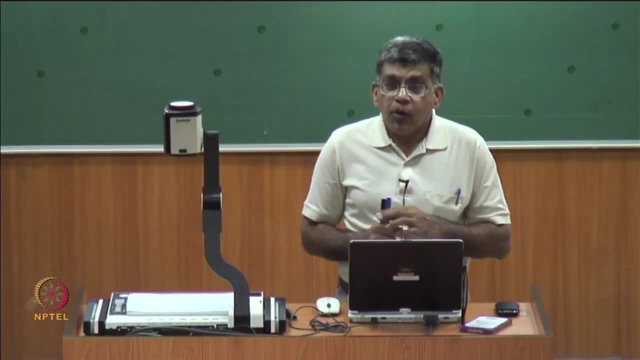 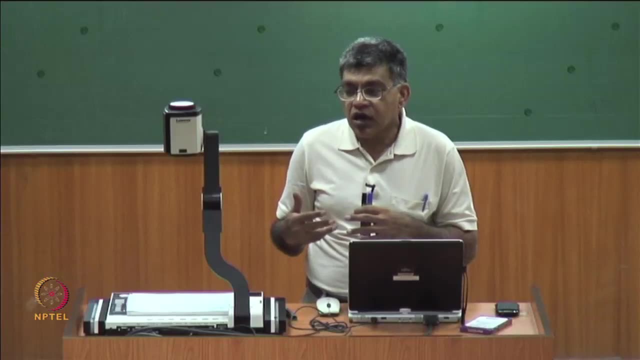 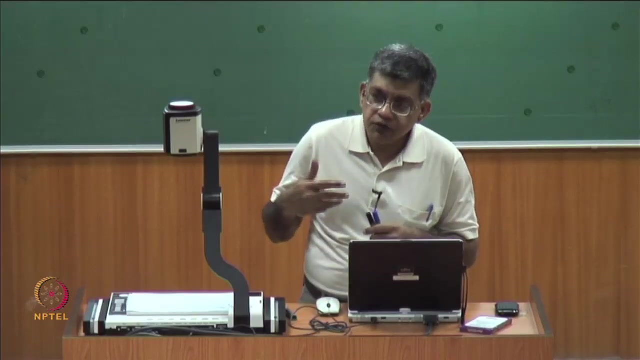 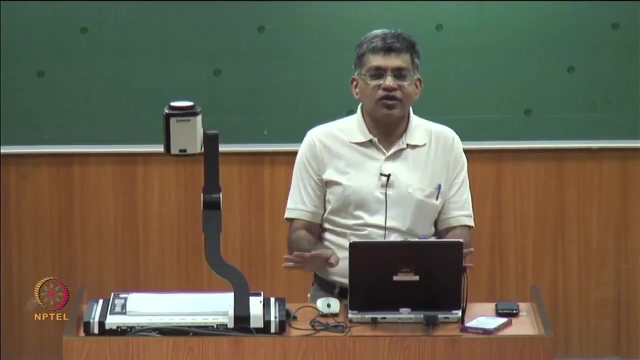 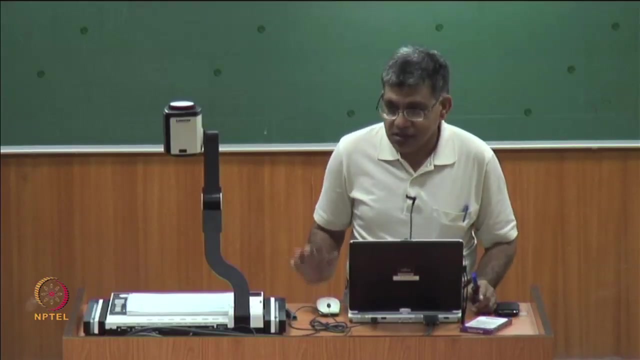 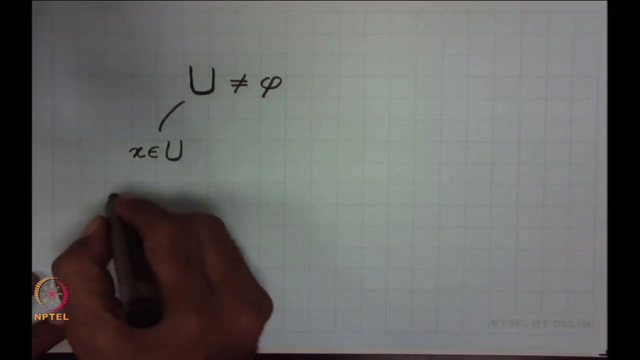 fashion, But properties of classes are, which essentially properties of subsets, and being able to describe properties of classes of subsets of this universal set is outside the domain of first order logic. So at the moment, so we are only looking at this, we are not look. So we are looking at essentially propositions, propositional. 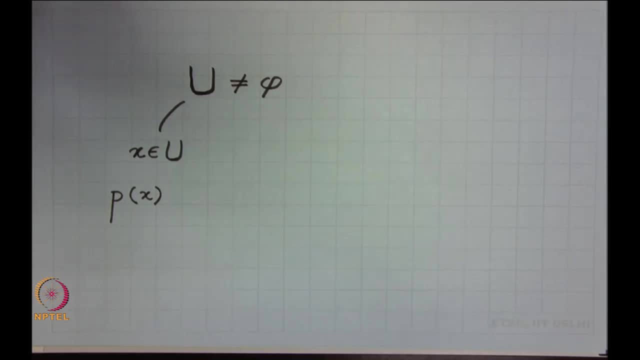 functions may be of the form p of x, But given subsets of u, we are not looking at propositional functions of this. So the moment this is outside the domain of first order logic. So we are only looking at propositional functions. 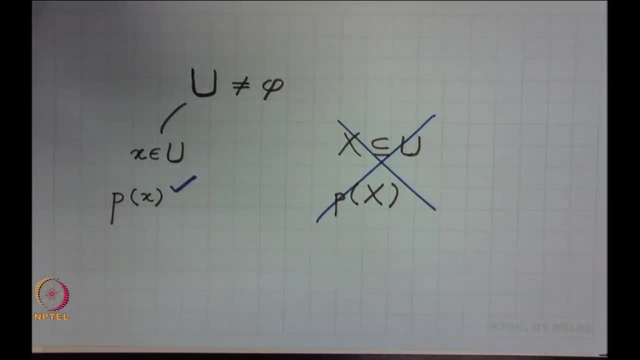 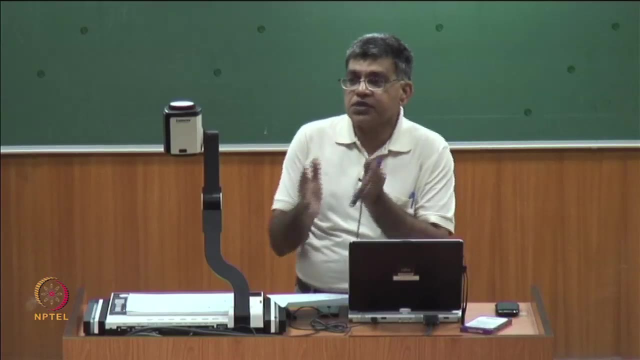 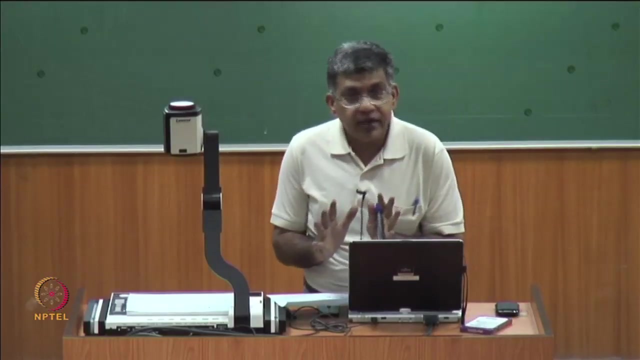 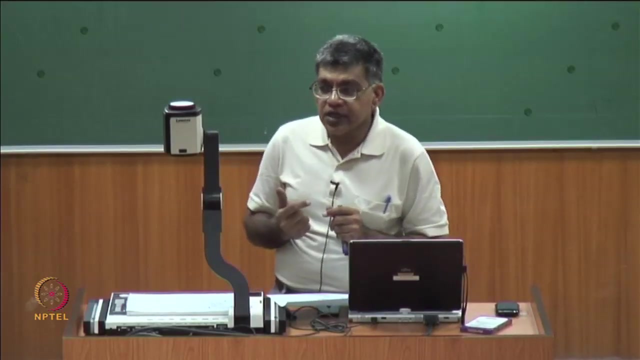 expressed in terms of individual individuals in the set and given that, given that there is a subset of u which might, for which this property p might be true, we might be able to characterize subsets of u that way, But we will not be able to characterize properties. 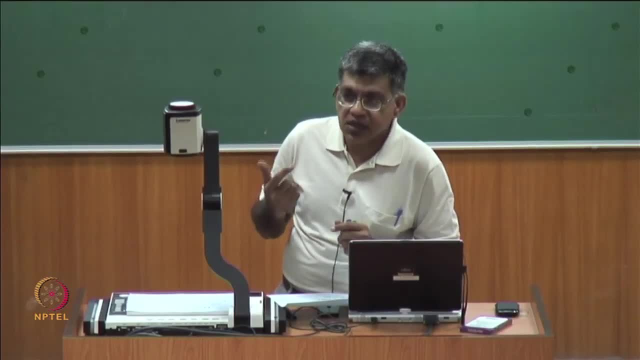 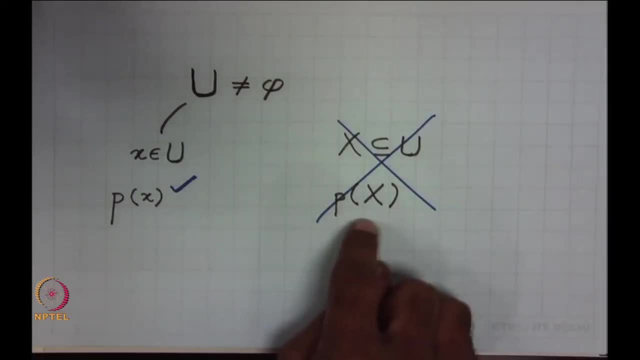 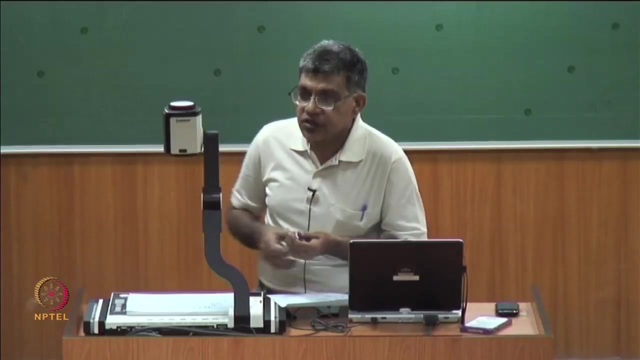 of subsets. of subsets I mean classes of sub classes of this set. So we will not be taking into account this. the moment you allow this also into your logic, then what you are doing is you are getting into second order. So, essentially, what then your domain of discourse really is then? 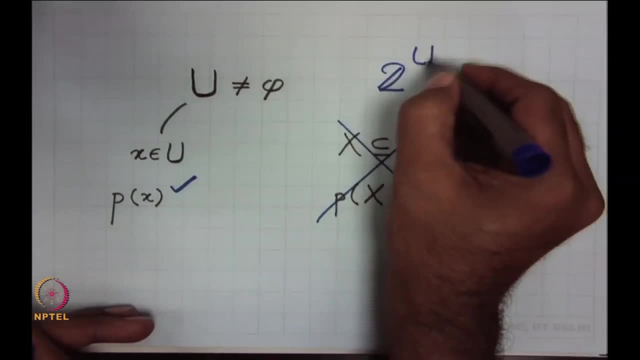 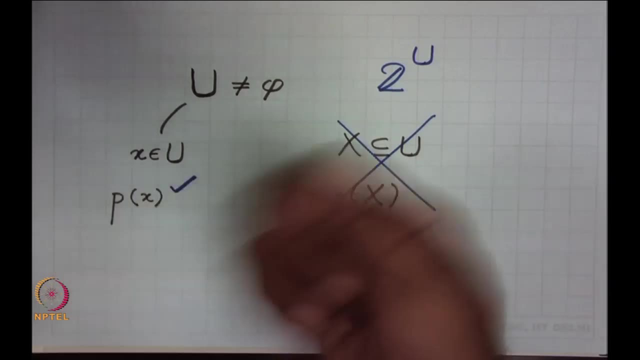 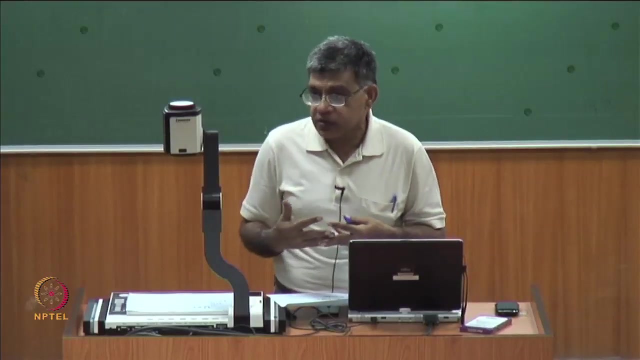 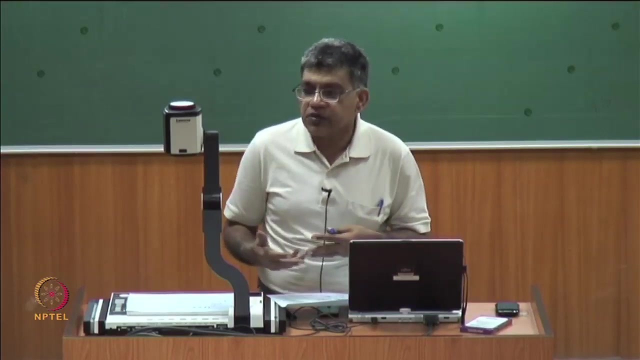 2 raise to u, and then you have 2 categories of individuals- Little x's and big x's- and then you can describe properties of these big x's also. So when you allow the description of that, then also along with the description of properties of propositional functions on individuals, then you get. 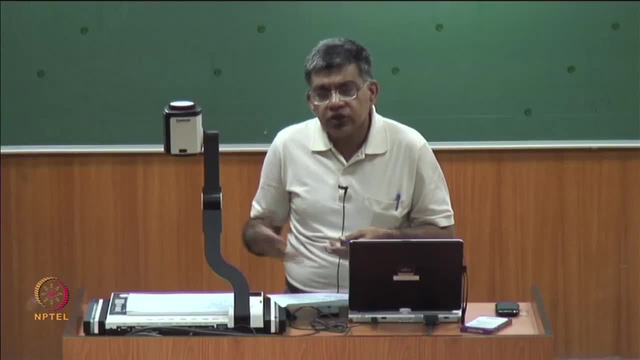 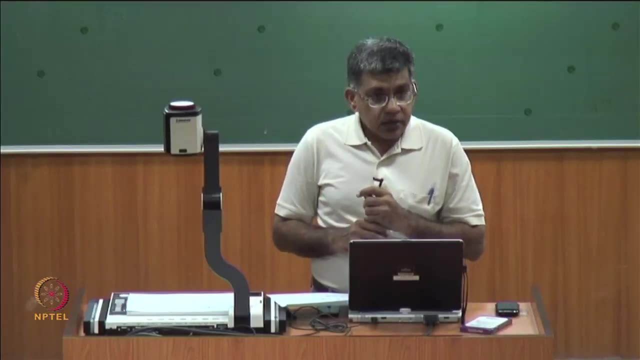 second order. The moment you go into 2, raise to 2, raise to u, you get third order and fourth order, and so on and so on. So Mathematics does use higher order also. I mean so second order and third order and fourth. 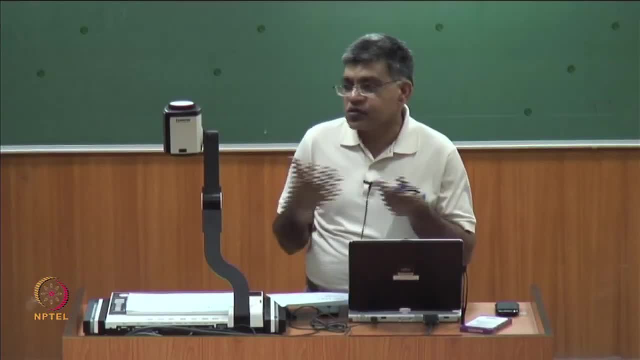 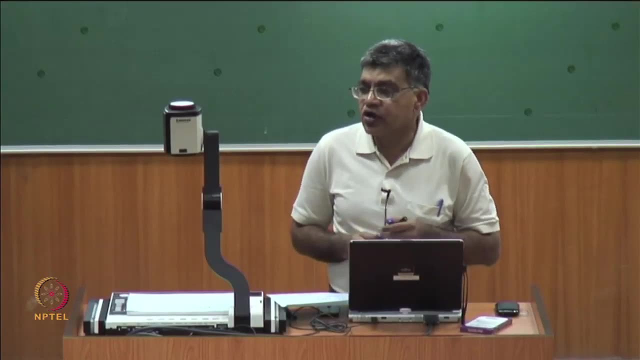 order. for example, various characteristics, properties of to by logical spaces are expressed essentially, they would essentially not fall in the domain of first order reasoning. So if you were to look at even the principle of mathematical induction, there are differences. induction, it is not really a first order property, for example, It is a higher order. 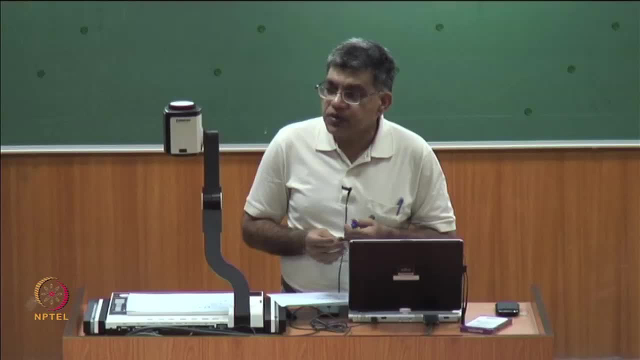 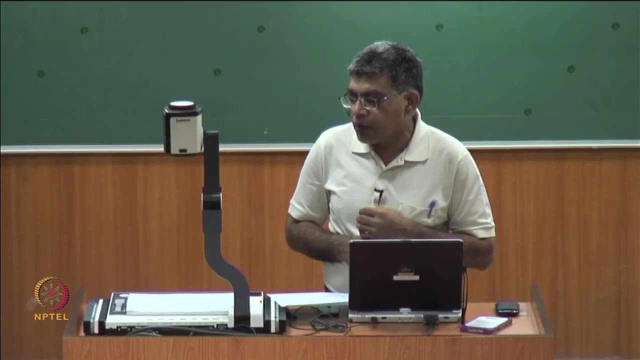 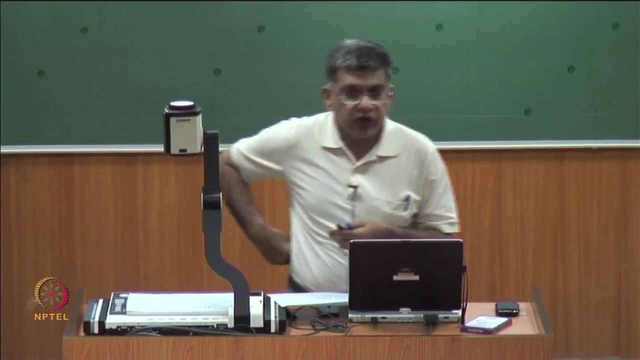 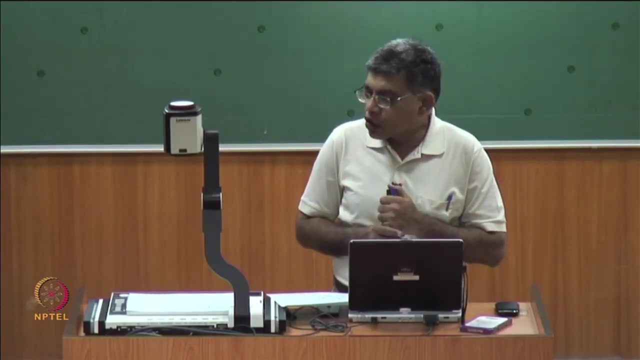 property, and so inductive principles in general are actually higher order. But once you have studied first order, at least the logical extensions to higher order are sort of obvious. the same kinds of quantifiers, quantification rules and so on apply, And so therefore you do not. so it is possible to actually look upon first order logic as 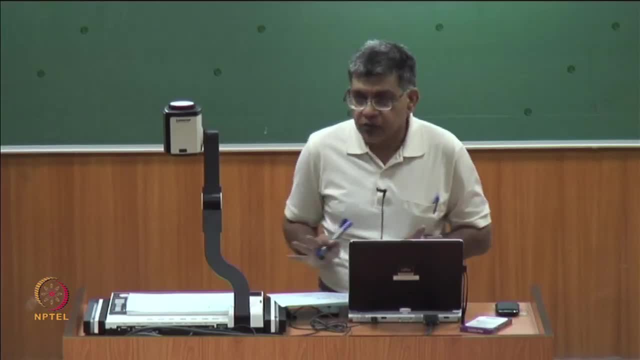 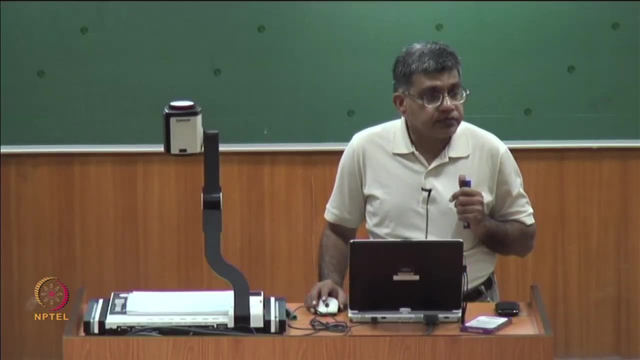 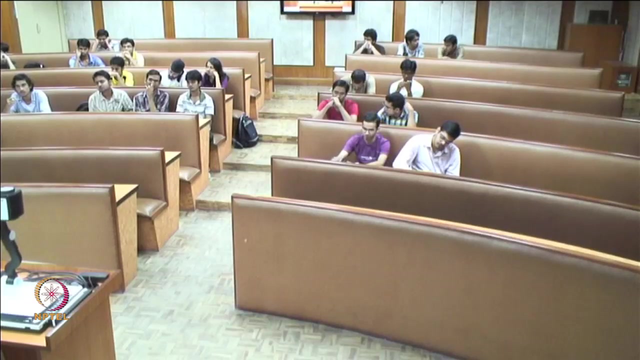 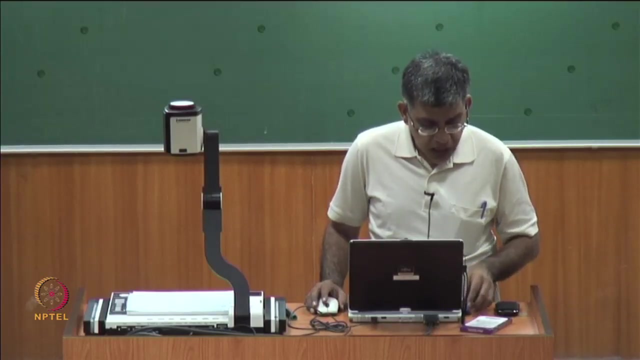 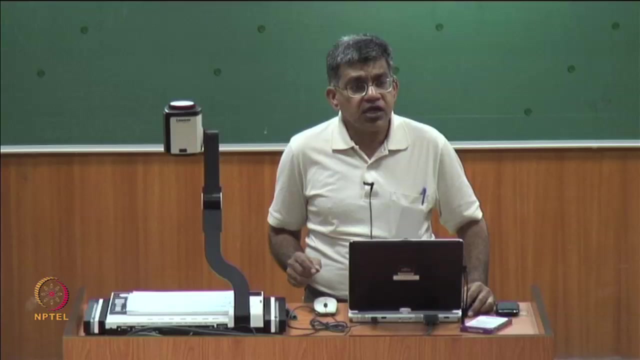 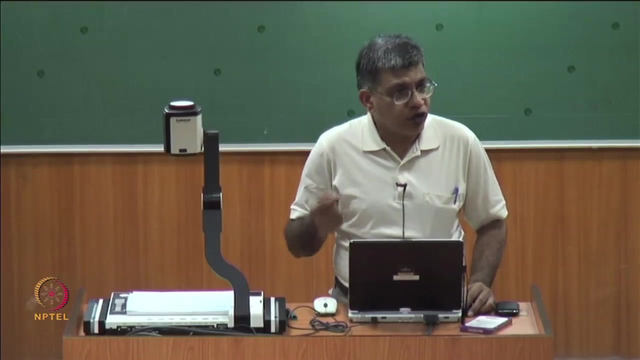 essentially being sufficient to describe most of mathematics. So that is what we are going to do. 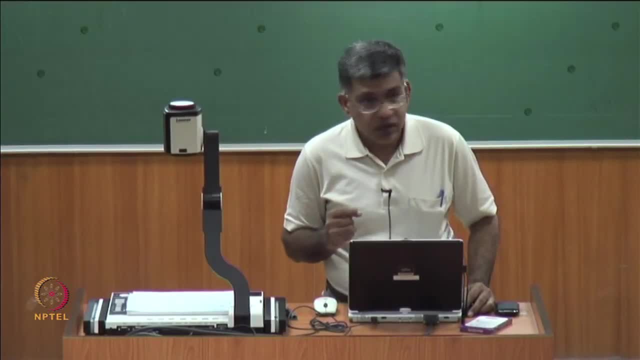 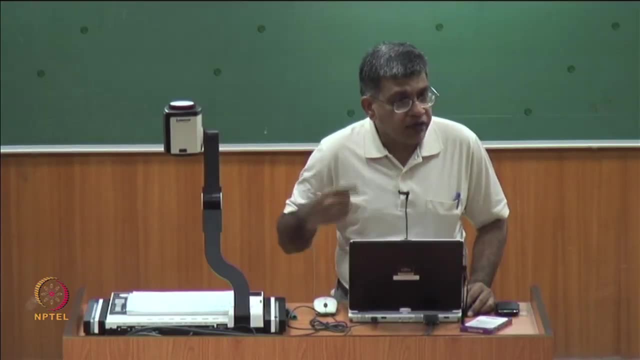 If, let us say, p is true of 0 and the fact that p is true of n implies p is true of n plus 1. Then p is true for all the naturals. let us say: but your induction principle. 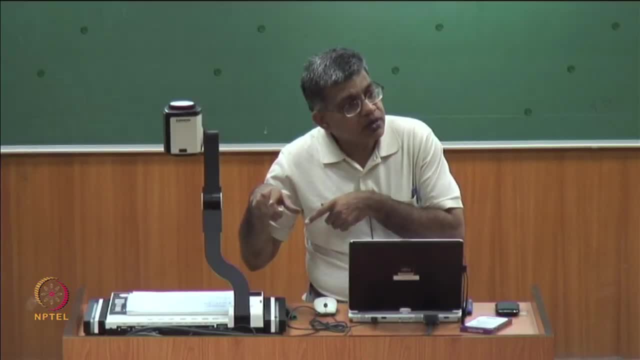 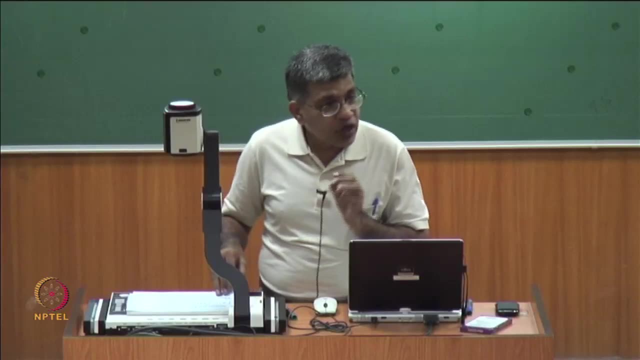 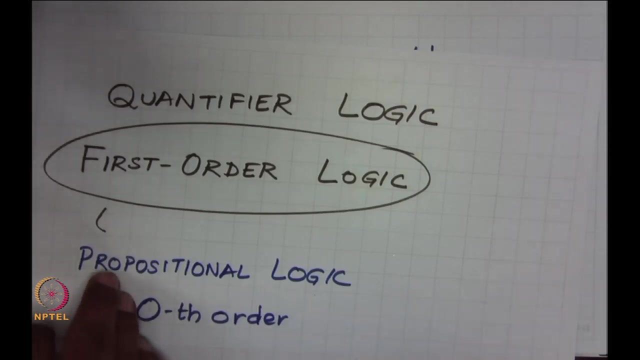 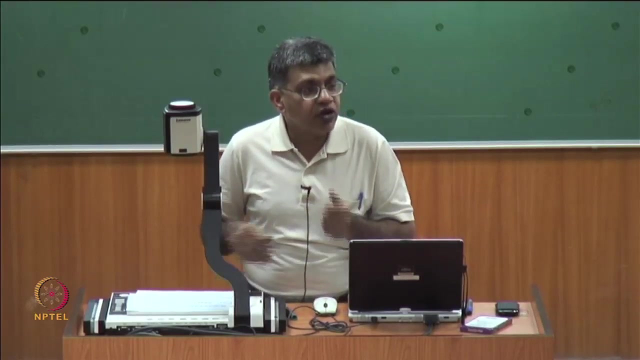 actually says this is true for all properties p. So in that sense you are actually quantifying over set of properties of natural numbers And you take any property of natural numbers that characterizes as a subset of the naturals. And when you are saying 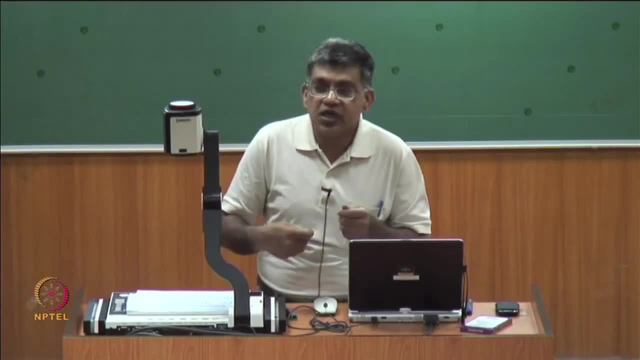 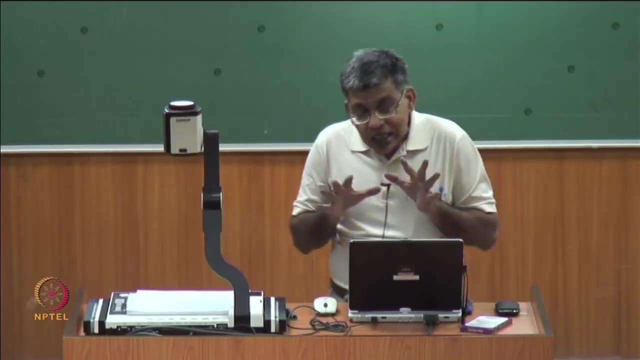 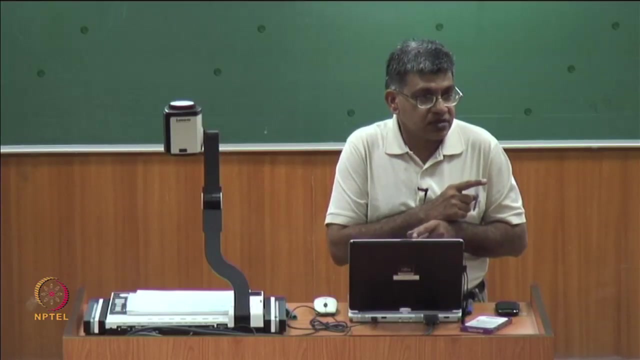 you are making a statement about all properties of naturals, you are saying for all subsets of naturals, And so your induction principle, the principle of mathematical induction, you are quantifying over all properties of individuals. In that sense, it is at least second order. what one can do, of course, is 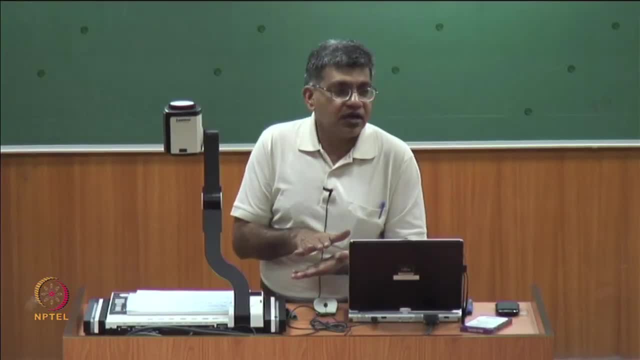 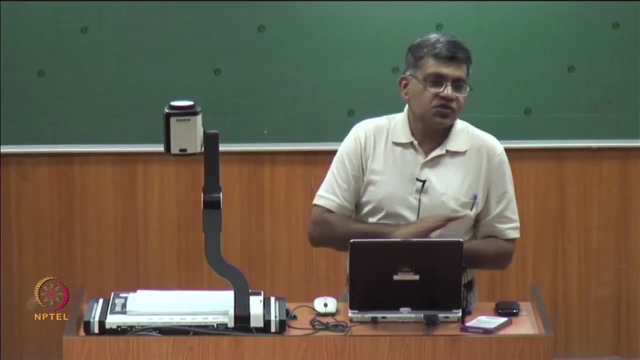 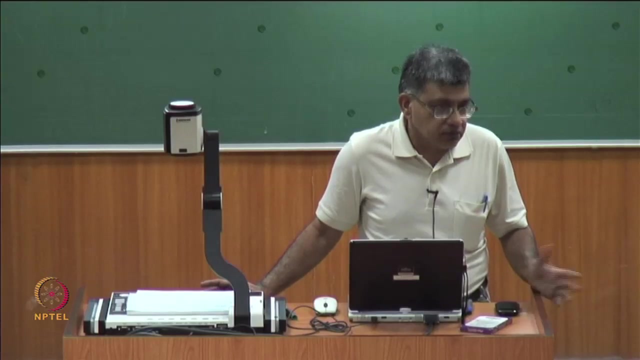 one can restrict ourselves to the particular order And say you take the principle of mathematical induction, restricted to first order. So that means you are just looking at properties of individuals and you just characterize maybe types of naturals. So induction otherwise is actually a higher. 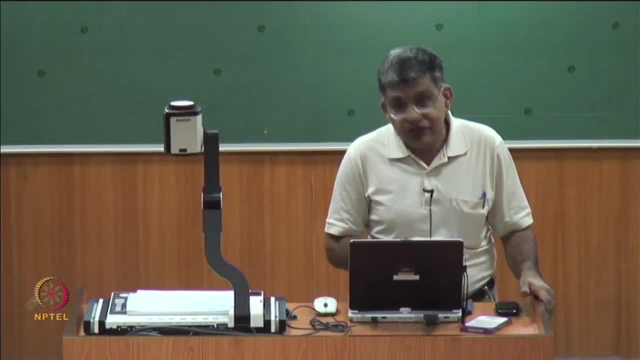 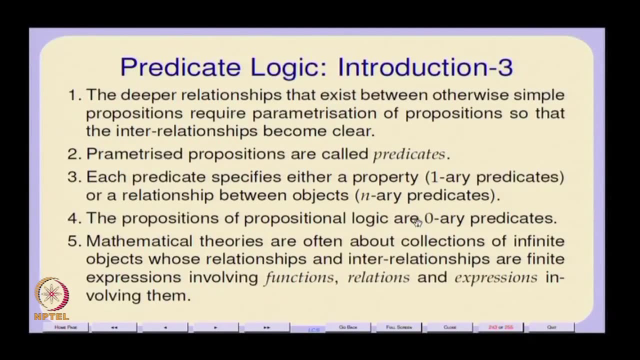 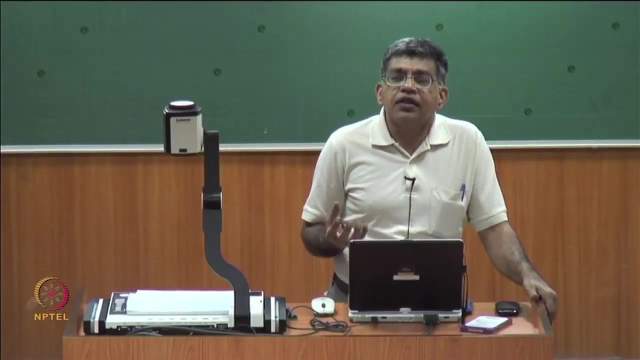 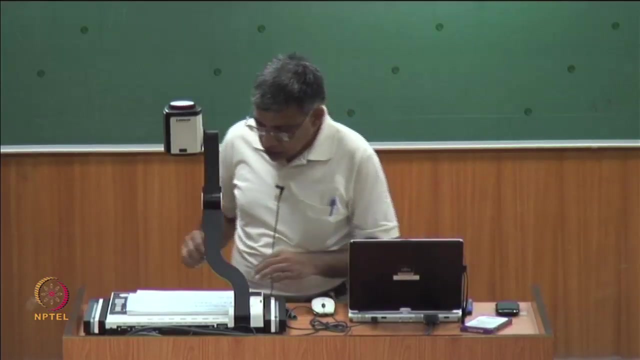 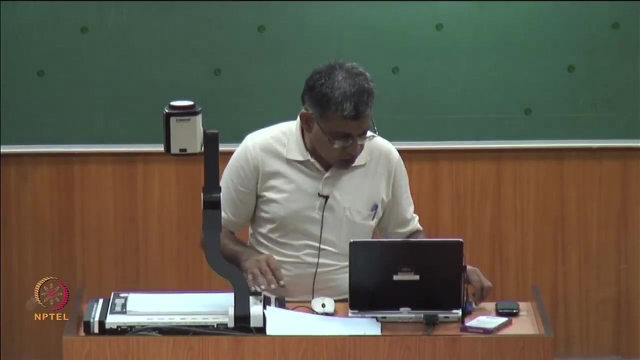 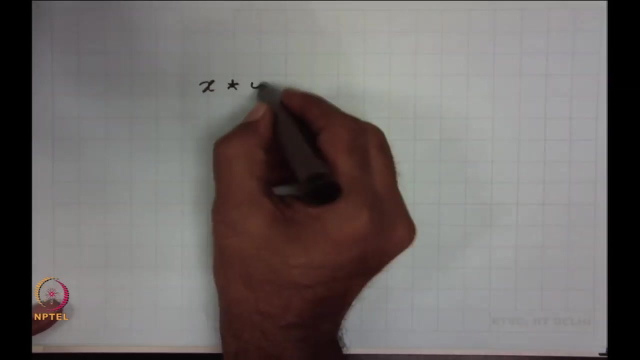 order property because implicitly, induction quantifies over all properties which satisfy this pattern. So that is another problem in general with mathematics text books and mathematics teaching is that this exact nature of quantification is never made clear. I mean So, for example, if you look at, say, the group theoretic axioms, I will just say x, y, z equals. 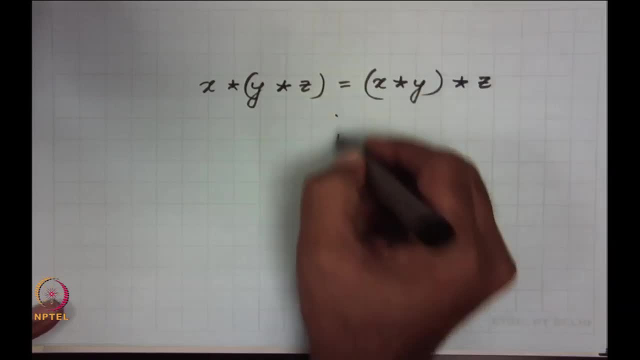 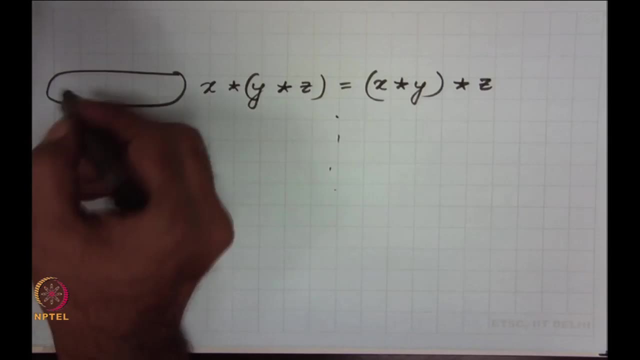 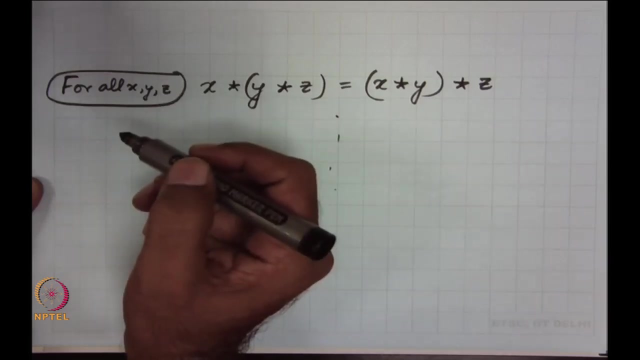 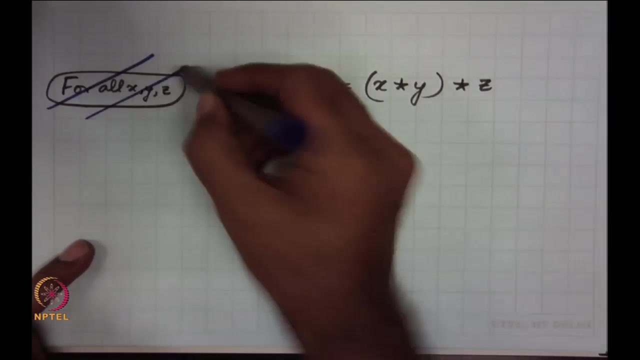 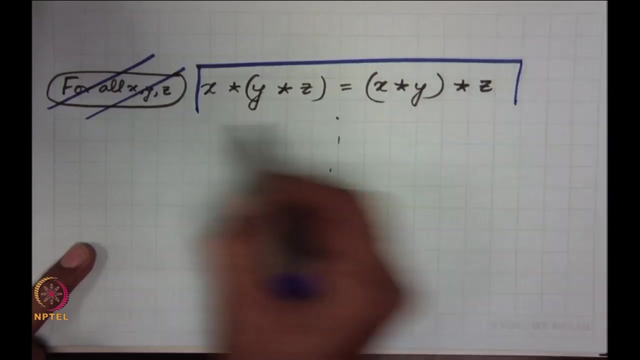 x, y, z and so on and so forth, But there is actually a quantification for all individuals: x, y and z. very often mathematicians just do not write this. many algebras will just write this in very much the same way in which we. 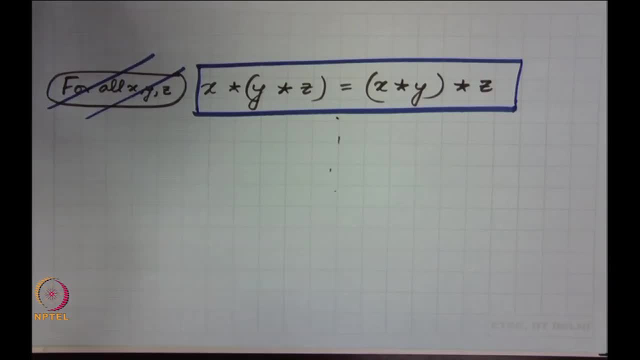 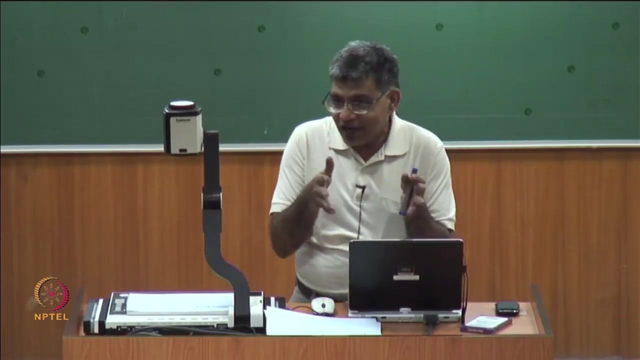 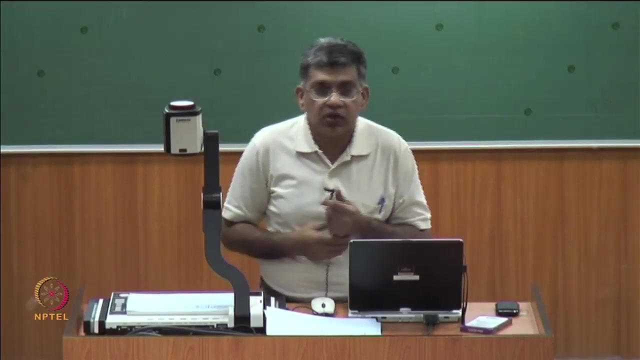 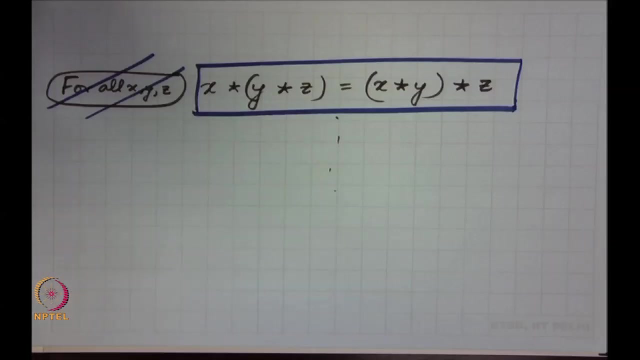 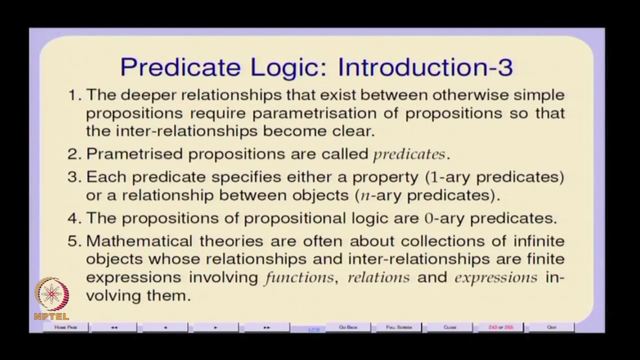 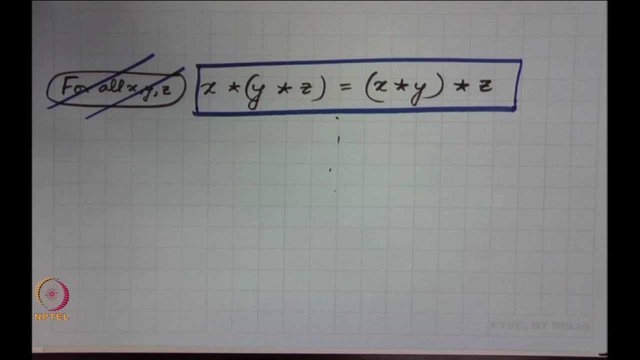 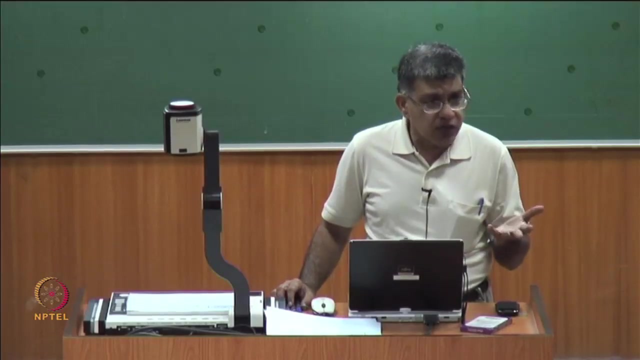 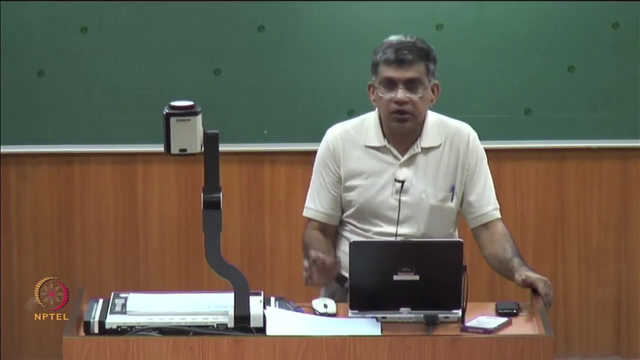 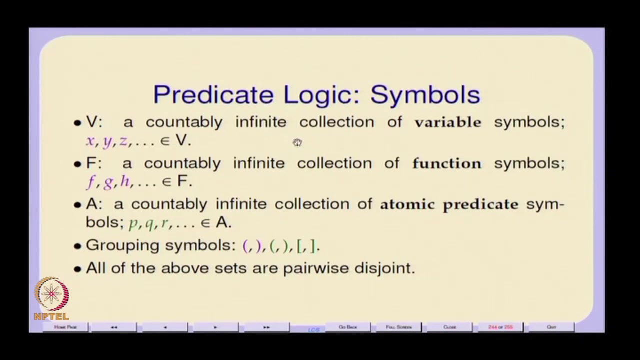 wrote rules of inference. We will start with the syntax of predicate logic. So, as usual, I have a set v of countably infinite collection of what are known as variable symbols. So, as I said, we are talking about propositional functions, very much like the way we move from, let us say, constants in very 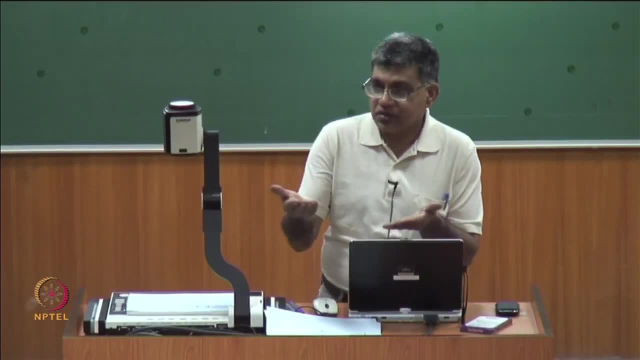 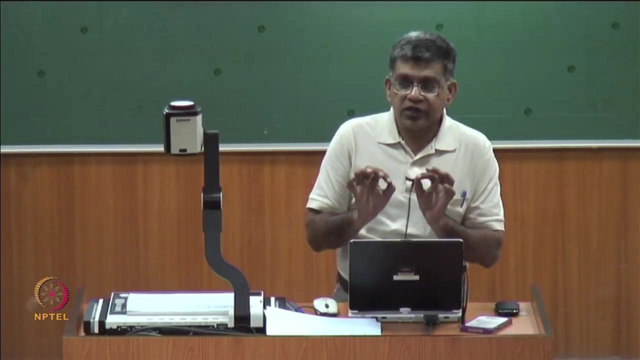 much like the way we move from arithmetic to algebra. I mean, just look at your the transition in your education from arithmetic to algebra. In the case of arithmetic, you had specific constants And you dealt only with specific constants. when you move to algebra, you actually graduated. 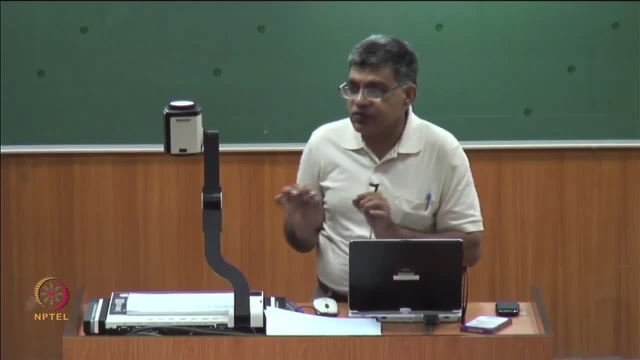 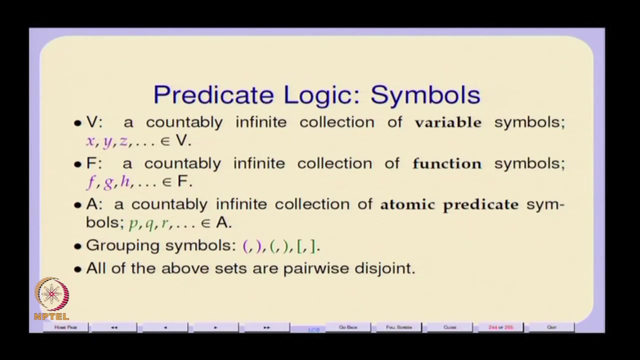 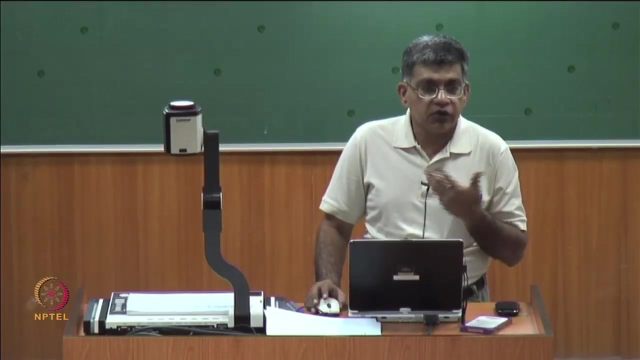 to using place holders without actually looking at specific constants. So the introduction of algebra naturally gave rise to the notion of variables. So when we graduate from propositions to predicates, which are just propositional functions, we are actually graduating from constants. So you require place holders and so this. so we will assume accountably infinite set. 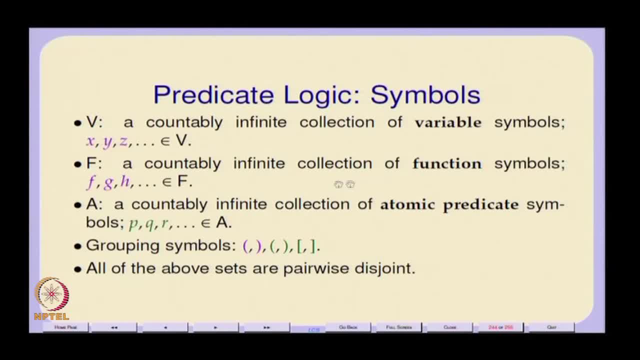 of variable symbols, And we will also assume accountably infinite collection of function symbols, because in any mathematical theory functions play a very important role. operations and functions will regard them as being. Almost any mathematical theory also has a collection of relations, and so those relations are what are going to be specified. 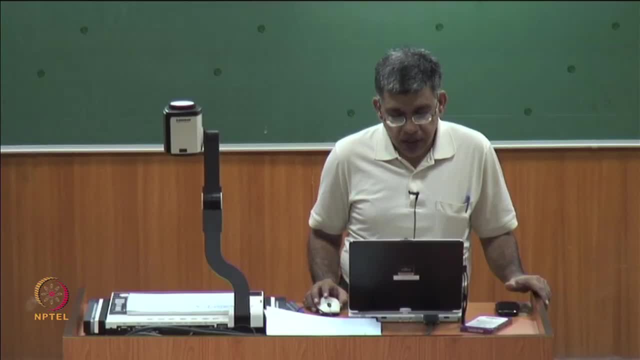 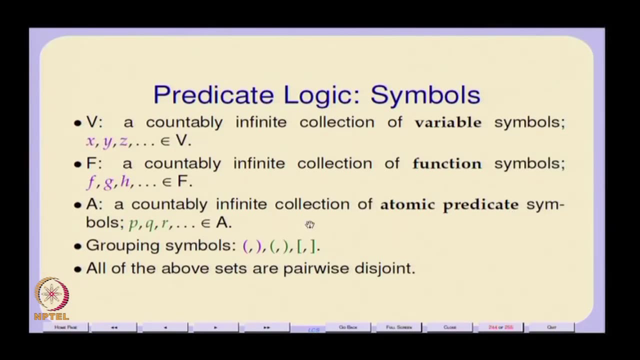 by predicates. So we have, So we will use these grouping symbols, and I have a peculiar problem that this scopes of unary operators and bindings is always something confusing, So I am using this square. 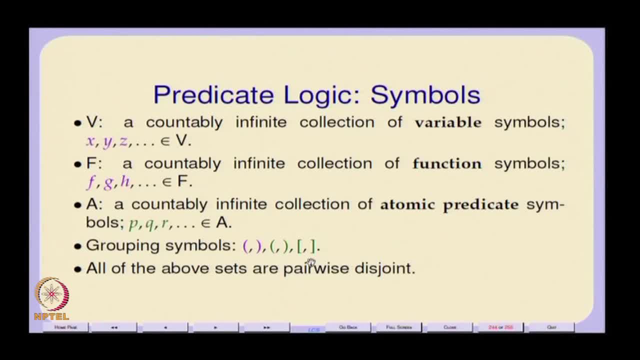 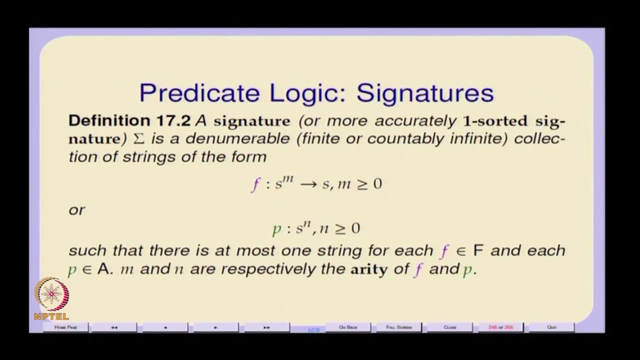 brackets. most logic books will not have this square brackets and, of course, all these above sets are pair wise disjoint. they are all separate sets And we will start with an algebraic notion. and the reason is actually historical and philosophical. if you look at- I mean historically speaking- if you look at the development of 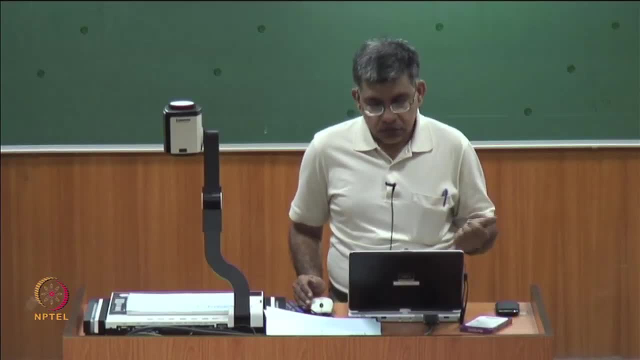 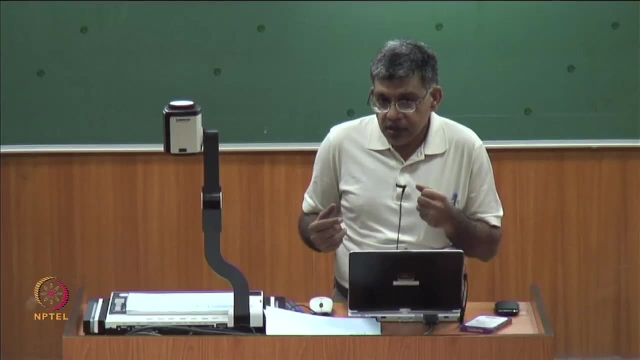 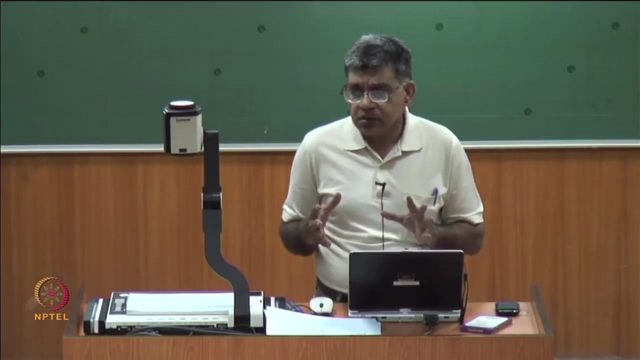 mathematics from India, for example. So the development of mathematics was essentially algebraic in nature, started with numbers, the place value system, arithmetic, and then went on to expressing various geometrical aspects, for example Pythagorean theorem, in a purely algebraic, as an 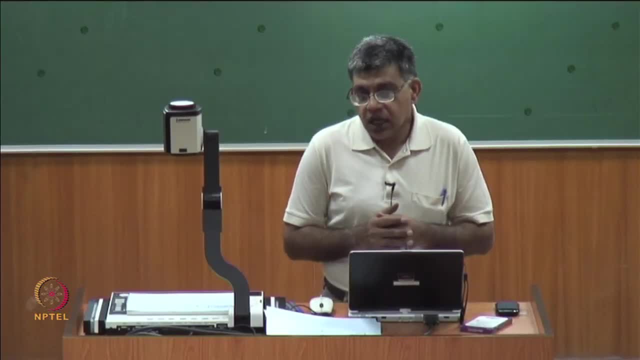 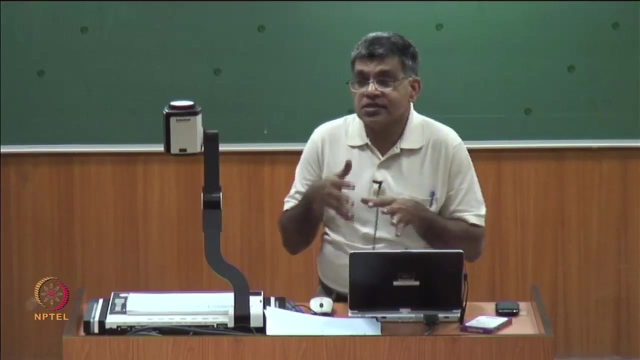 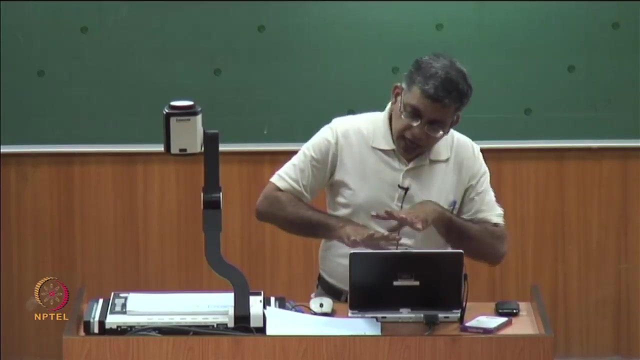 equational form as an identity, And then trigonometric relations and so on, as essentially, as in an arithmetical or algebraic form you can, any kind of algebraic form is also, it also has a certain syntax and therefore you can think of it as a linguistic form. So what actually pervaded most of ancient? 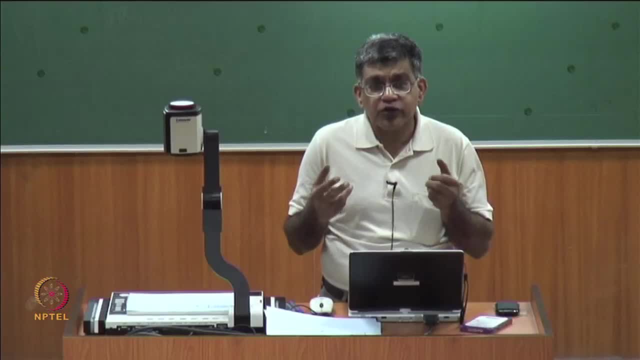 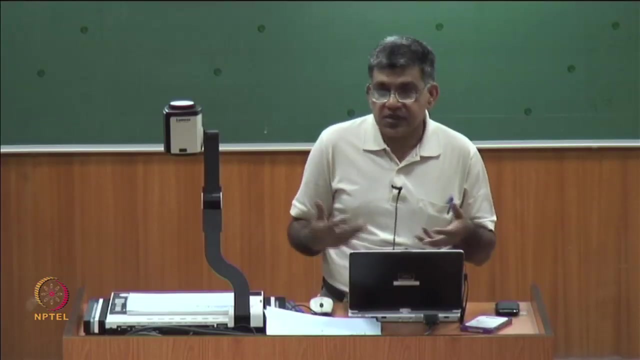 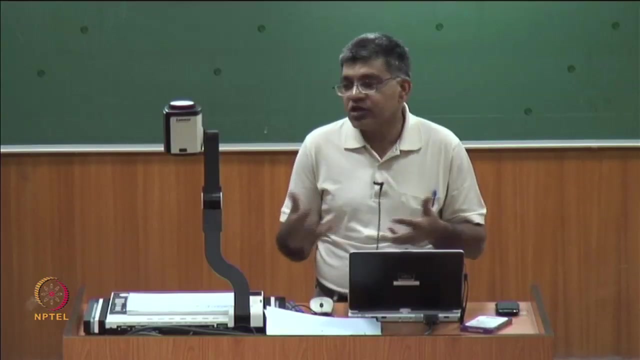 Indian mathematics is a high proportion. So that is the definition of algebraic reasoning. So, and therefore linguistic reasoning also. So if you look at the formalization of Sanskrit by Panini, that is essentially like defining a formal grammar and formation rules, very much in an algebraic sense. 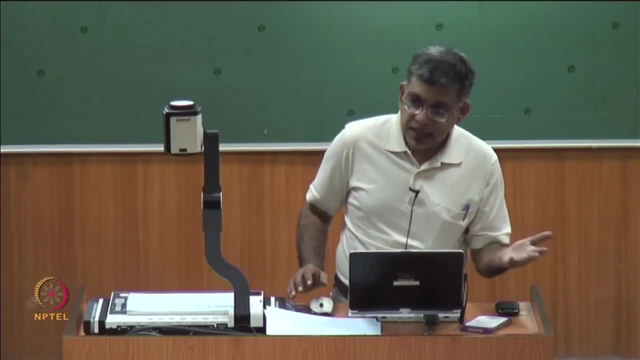 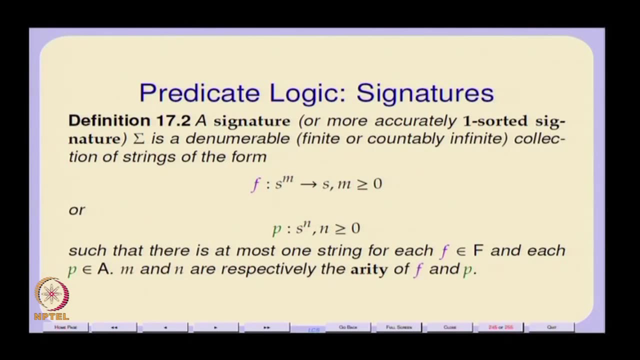 On the other hand, if you look at the developments in Greek mathematics and starting from essentially starting from Egypt And then moving on to Greece and then coming back to Alexandria, I classify all of that as essentially Greek mathematics. the primary problem there was not of numbers and symbols and manipulation. the primary problems there. 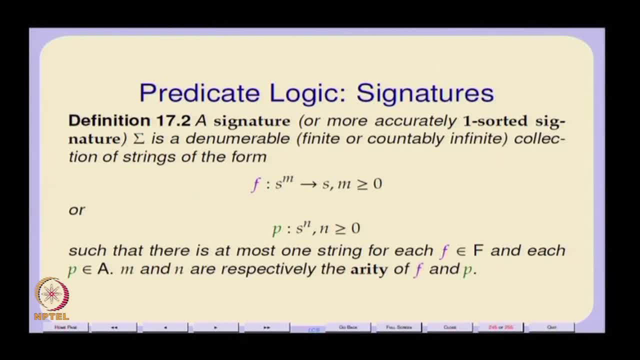 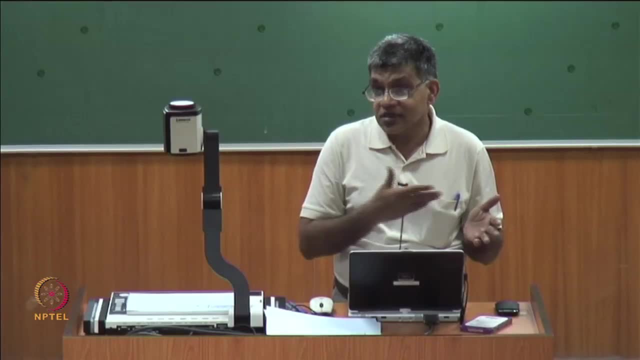 were all of a geometry nature: being able to predict when the Nile is going to flood the planes. being able to predict the course of the Nile river, for example, being able to do triangulation, being able to walk across the desert and get some navigational aid using the stars, and 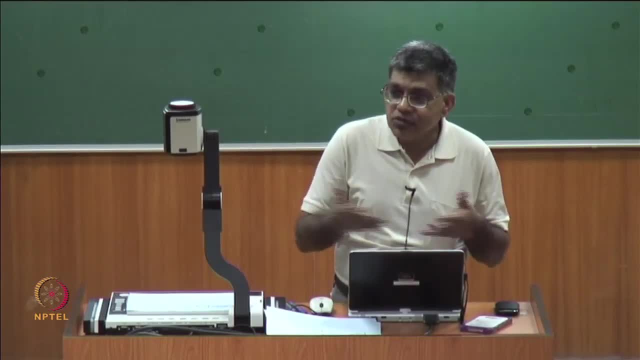 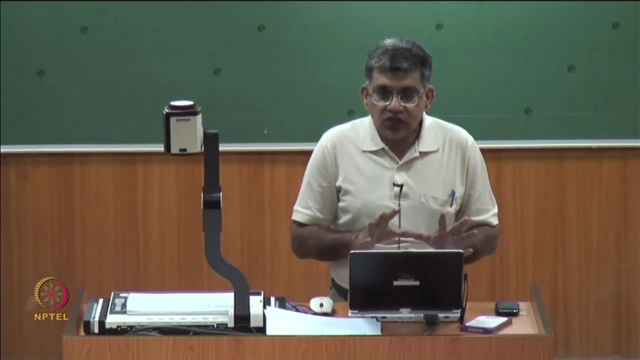 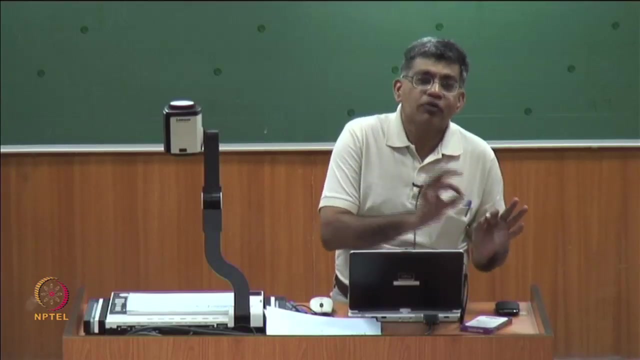 so on and so forth, using the sun in some geometrical fashion, the angle of the sun, and so on. So the entire development of mathematics actually was divorced from the. there were numbers, of course, but it was primarily geometric in nature: the angles, lines, straight lines, planes, heights, distances, and so on and so forth. and 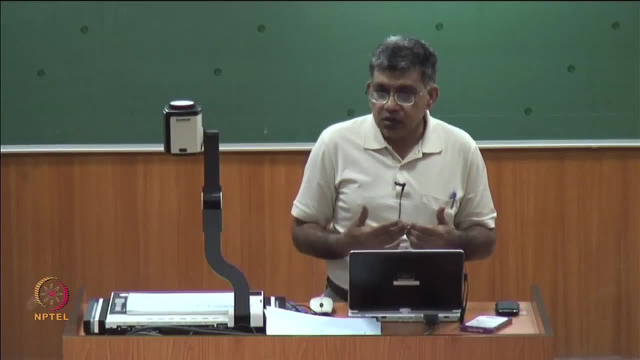 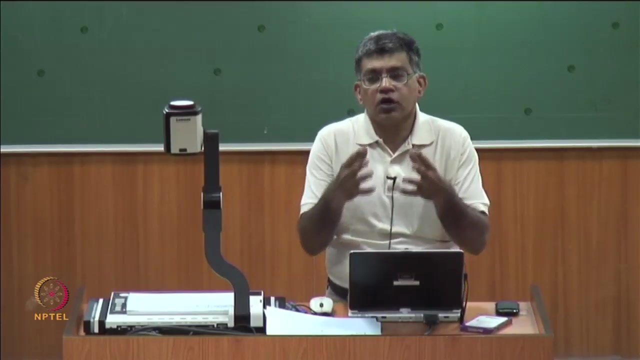 even up to the 11th or 12th century. if you look at the problems of Greek mathematics, including the Diophantine equations and so on, which we see in an algebraic form nowadays, most of their solutions. for example, how do you solve quadratic or cubic equations Most? 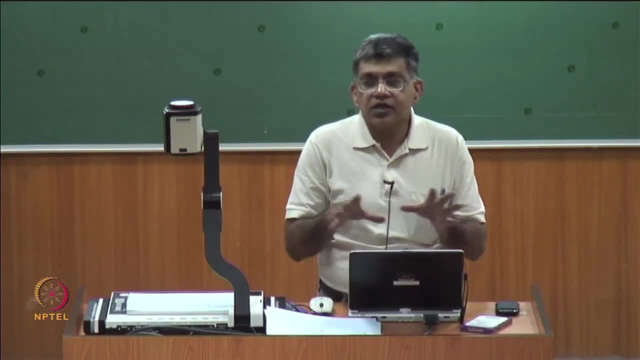 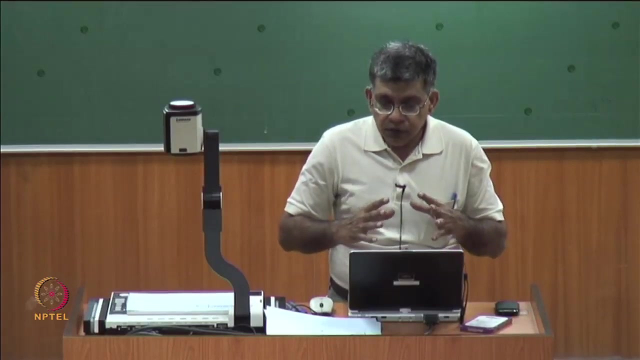 of those were expressed. quadratics were expressed in terms of areas and cubics were expressed in terms of volumes. So this, what we would regard as a simple cubic equation to be solved, the Greeks would actually imagine volumes of rectangular cuboids and cubes placed in certain fashion or removing. 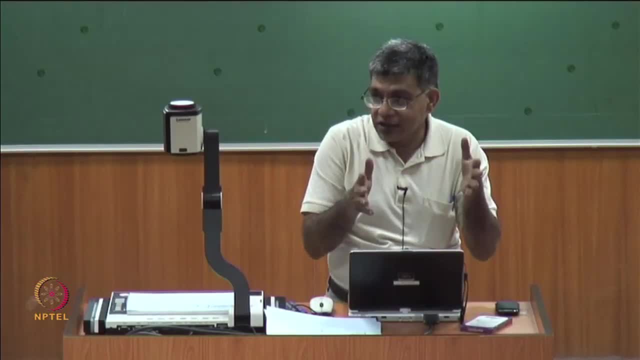 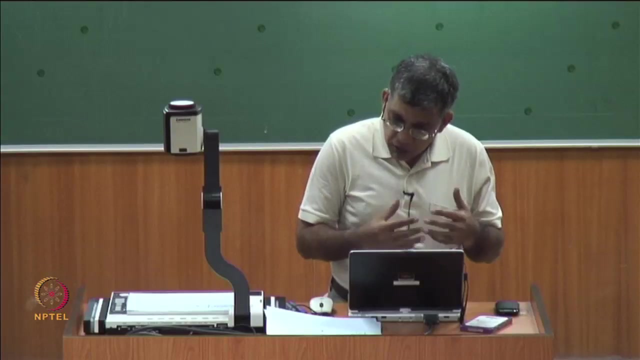 sub cuboids and sub cubes from other cuboids and cubes. So subtraction was essentially removal of volumes and then their resulting volume, and so on and so forth. So even the solution of equations had an absolutely geometric flavor to it, and it was always. they always drew diagrams in some. 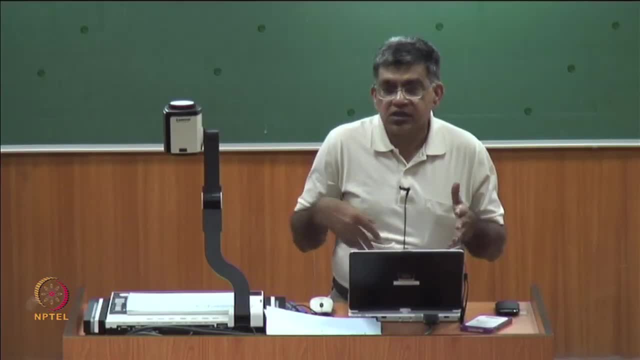 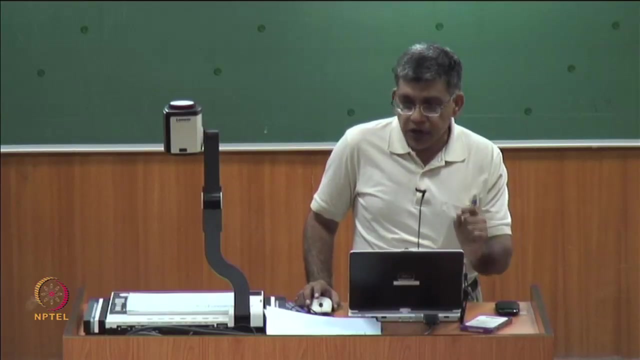 kind of perspective mode or in some kind of isometric mode and actually try to reason using volumes and areas, and even when they have to deal with second degree equations and third degree equations. So but the whole point was that with Descartes, 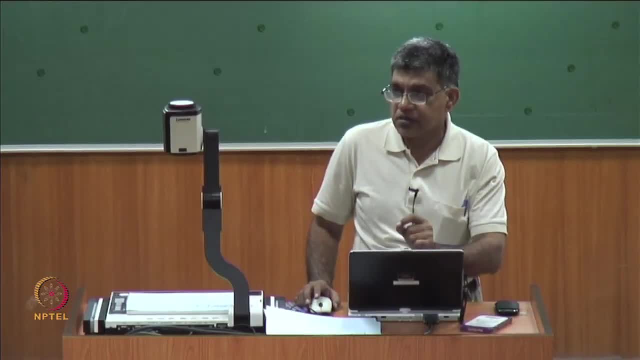 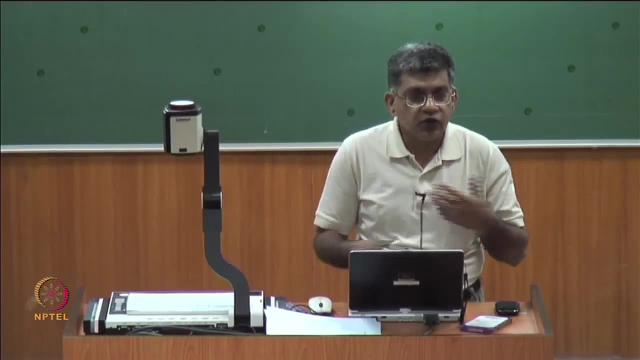 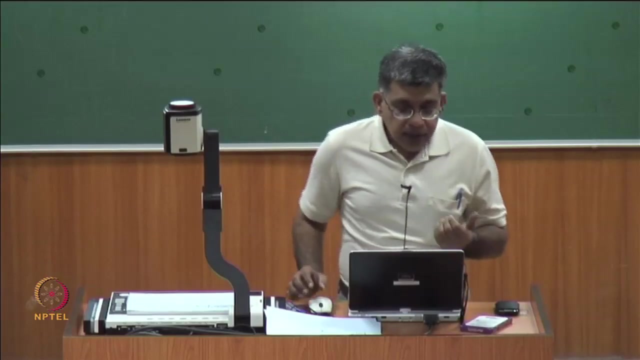 actually the whole of geometry got algebraized. Once you have a coordinate system and the notion of a point is an ordered pair of real numbers and so on and so forth, and then you use the properties of algebraic properties of real numbers, you have algebra is geometry. Therefore, in a certain sense, the interactions, 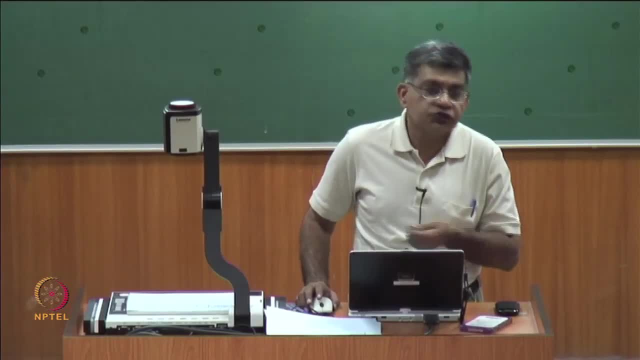 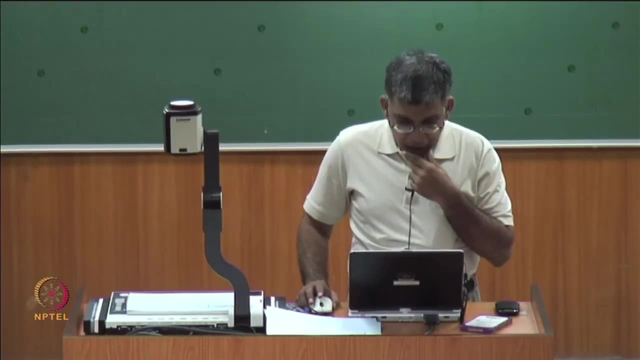 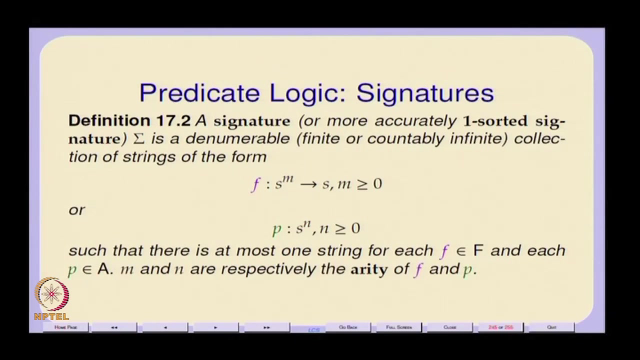 between algebra and geometry. so if you take the development of differential or integral calculus, that is also an algebra or geometry, essentially, of course you like. So algebraization is part of linguistics and therefore if you are looking at a formal language development, we will look at all mathematical theories also in some algebraized form, right? 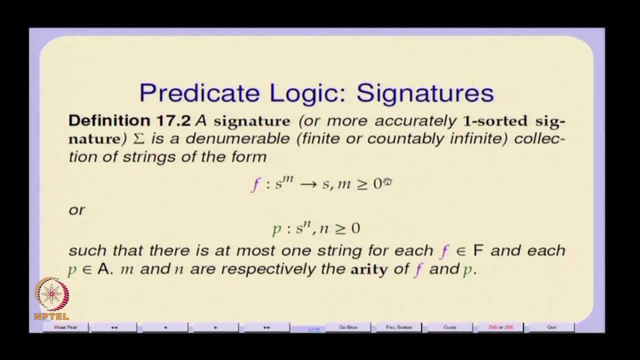 So we will look at signatures. so any mathematical theory, we will think of it as containing a signature. So this signature essentially gives you finite or infinite collection of function symbols with their rarities. So this essentially is a specification of their rarities and these predicate symbols have their 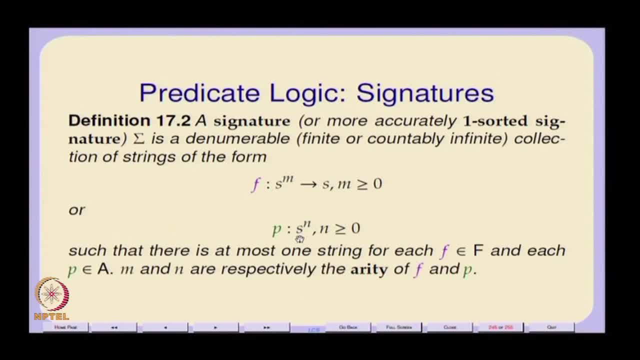 rarities specified by So. S is just a formal symbol for a sort, so there is a sort. So what we are looking at are one sorted signatures. If you were to look at a typical programming language, a typical programming language can be thought of as a many sorted. 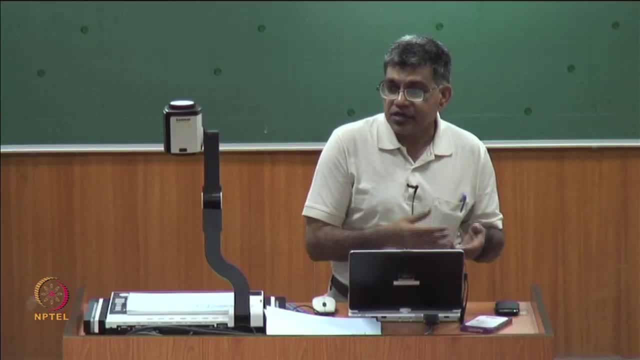 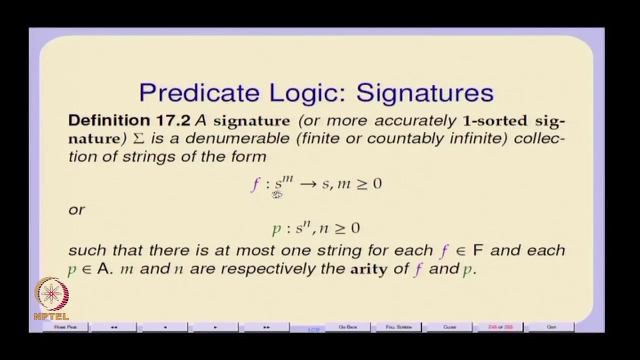 algebra. So there are several sorts, like booleans, natural integers, reals, strings and characters may be, And on these, and then there are operations between these sorts. So then, instead of using a single symbol S, we will use many symbols- S1, S2, S3- to specify essentially the signature. 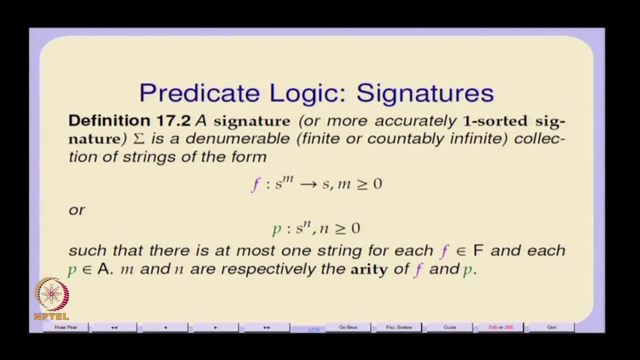 of an algebraic system, And this notion of a signature is exactly what your modern functional programming languages also adopt. I mean, there is a, So they have this notion of a sort. So, for example, ml or camel or haskell has this int. 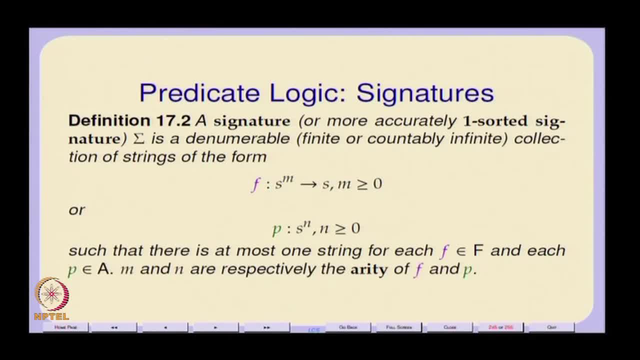 and bool and char and so on and so forth, And you specify signature essentially in terms of these functions and predicates, these function symbols and predicate symbols, by specifying essentially the rarities right And the sort of the domain and the co domain in the case of functions, in the case of predicates. 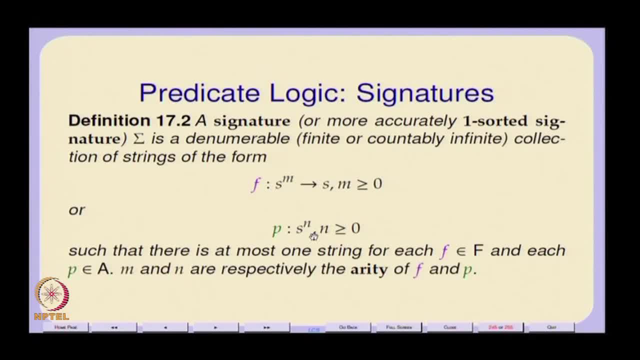 of course the you can. they are thought of in programming languages as functions which take you to bool, booleans, right? So that is, in that sense there are only functions there. So we will look at this. So we will assume that you got some signature specified for each function symbol and each predicate symbol. 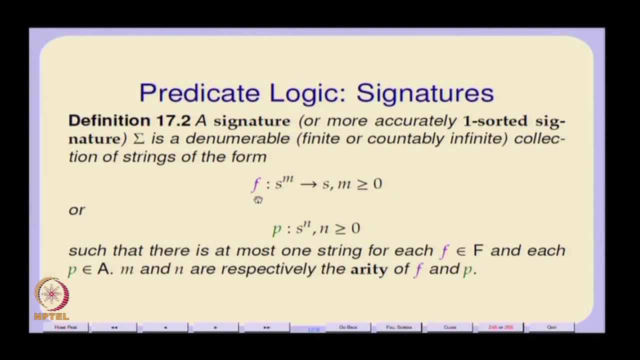 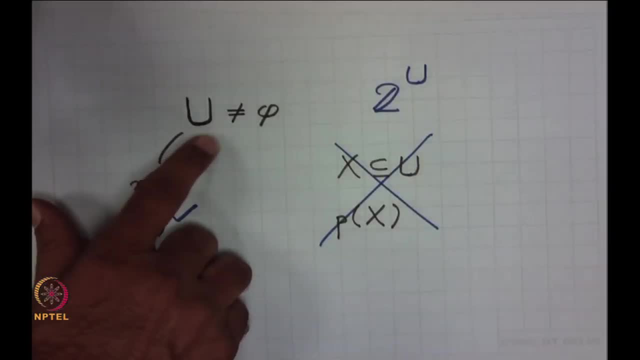 And we will assume that there is no conflict. So, for every function symbol, there is a unique string specification. So, in terms of the sort, and we are looking at one, sorted signatures, which essentially means in our mathematical description, we are looking at this, we are looking at this you. 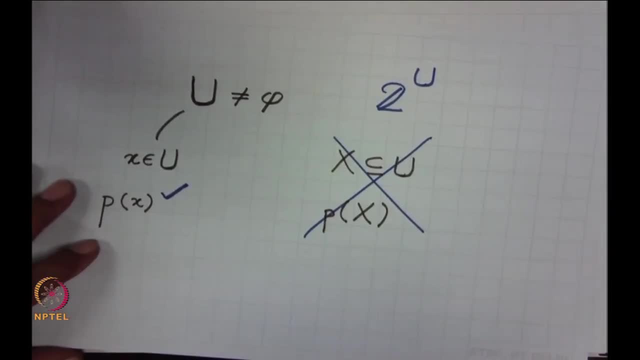 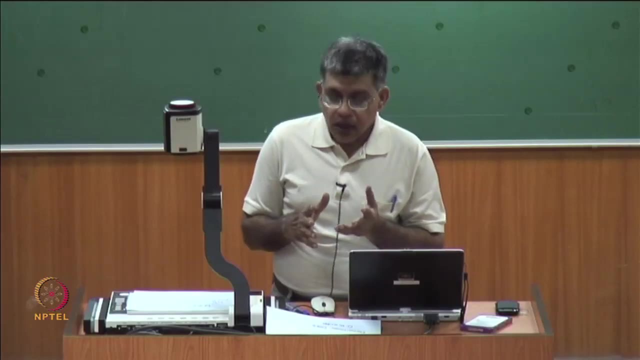 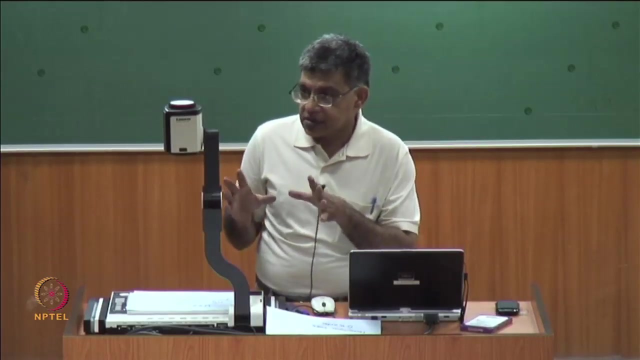 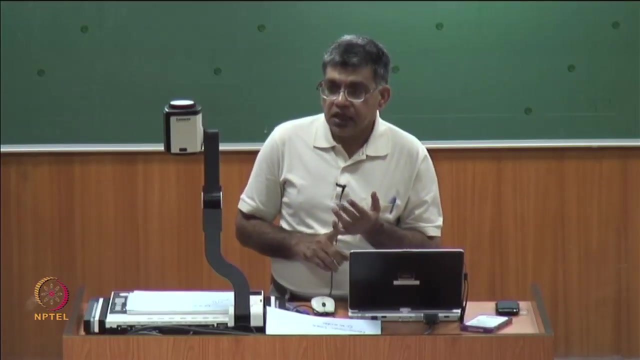 as a single sort. The generalization to many sorted signatures is not very hard. one could do that too, But it just becomes more complicated and tedious. So, but there is, there are no technical problems with the generalization. But there is also another thing that it is possible to take. 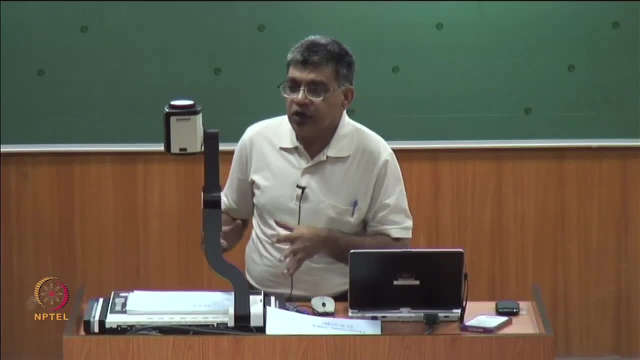 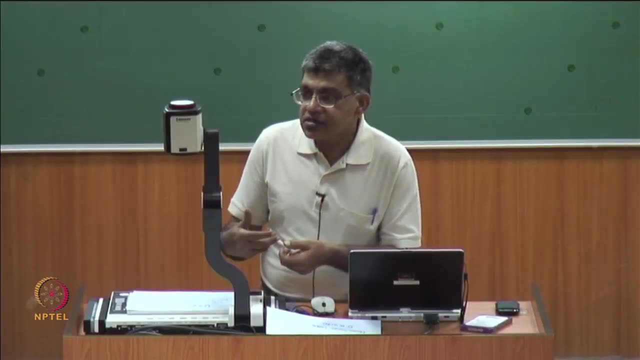 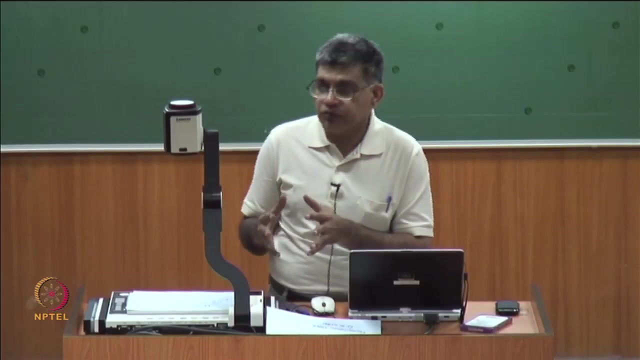 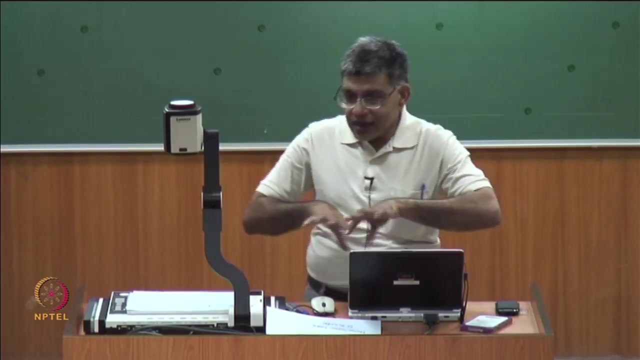 the many sorts that you might have put them all together and call them a single universe And have distinguishing predicates as for the membership in the various sorts. So you can have membership predicates, essentially for the to distinguish between elements of various sorts. So they would, if you had a collection of disjoint sorts, then you use 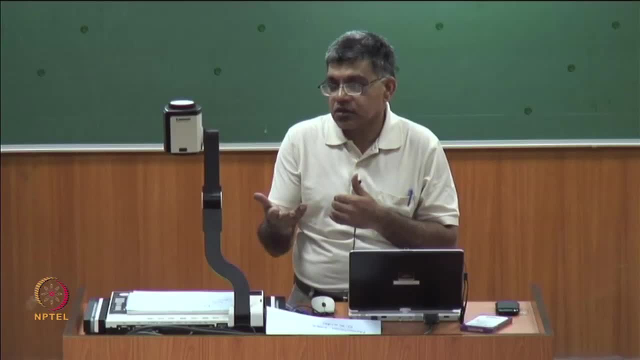 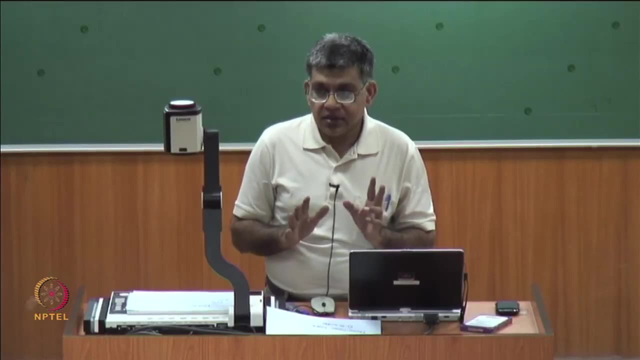 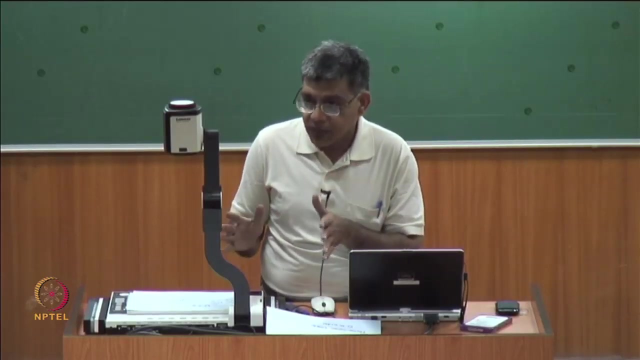 one predicate to essentially specify membership in a sort. So then, the net effect is that, either case, your many sorted algebra becomes tediously complex, complex, But even many sorted algebra, given a finite number of sorts, can be described through one sorted algebra, by just adding these extra. 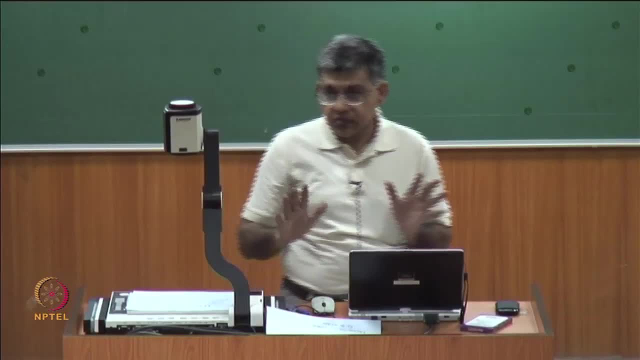 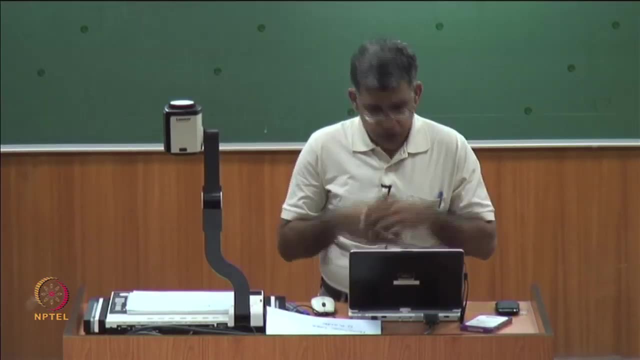 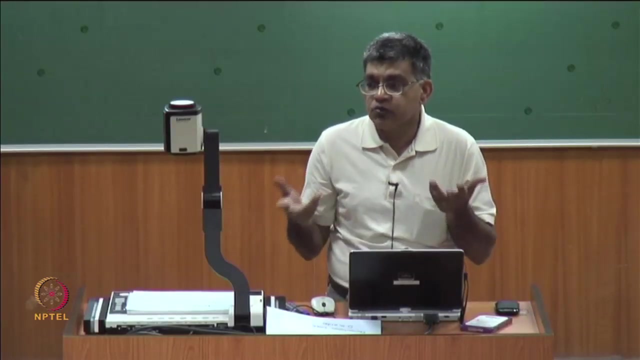 membership predicates in the signature. So what I, for example? the simplest thing is to take integers and Booleans, put them together, take a disjoint union of them And just have one predicate which specifies whether some an arbitrary object taken from this thing is either Boolean or integer, And have these two. 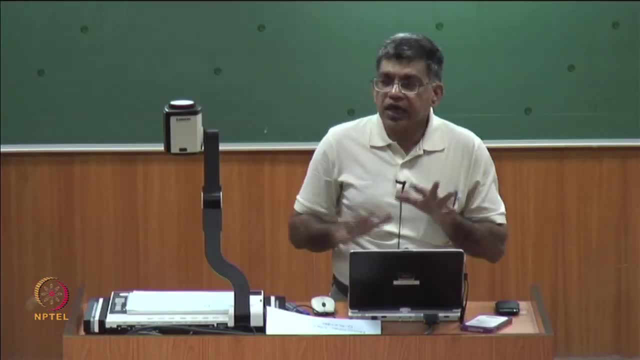 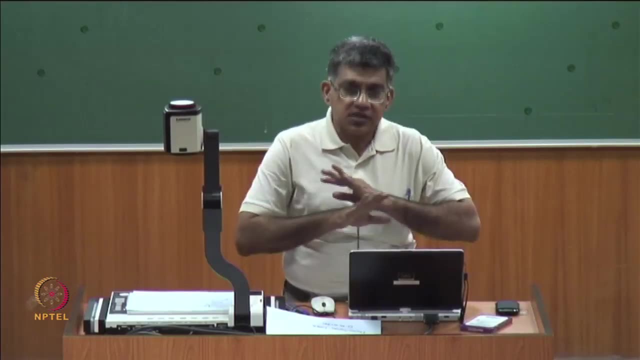 predicates, integer something and Boolean something And you can actually everything that you can do with many sorted- at least a finite number of sorts you can do in a one sorted case. So it is sufficient for us to consider a one sorted case. So that is important. 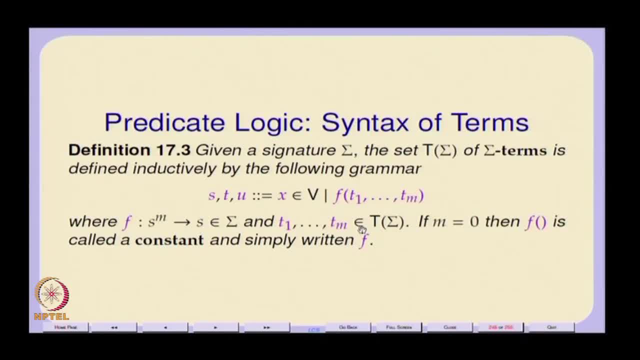 And then, of course, we have this notion, we have this, we have a term, we essentially define a term, algebra. So, given a signature, sigma, and we will just assume a one sorted signature, We have a set of terms. sigma terms is defined inductively by this grammar and I will use this violet color essentially to for terms. 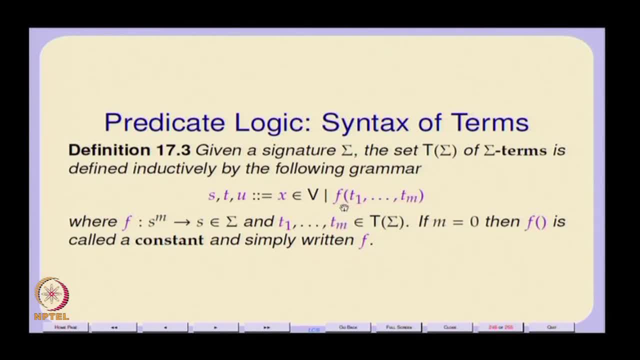 here. So if f has a signature s, m arrow s, then f can essentially take other terms as parameters, and this is an inductive. this is an inductive definition in which I have gone beyond the usual b n f grammar by specifying also other things in short hand, So s t u. 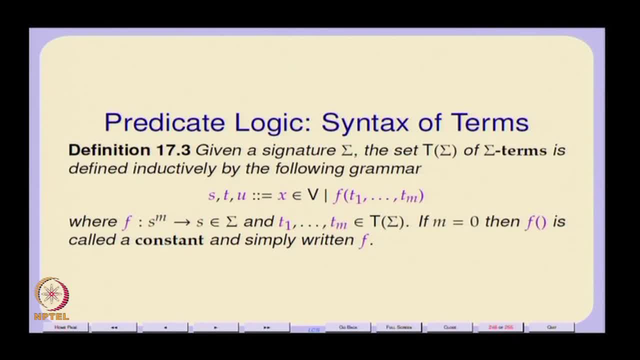 are like are typical example, are typical members of terms. So I will use these symbols, like s, t and u in violet, for to denote terms. this x equals, x belongs to, v essentially says that all the variables are terms and so on. So they of. 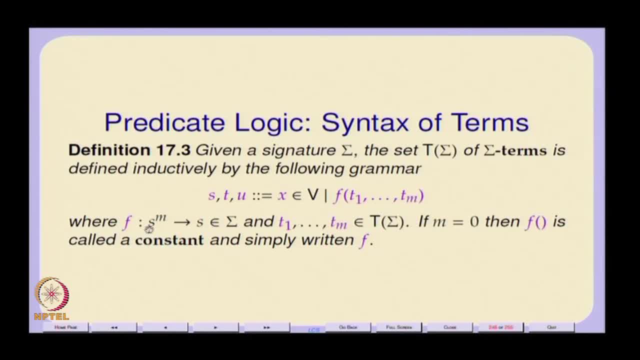 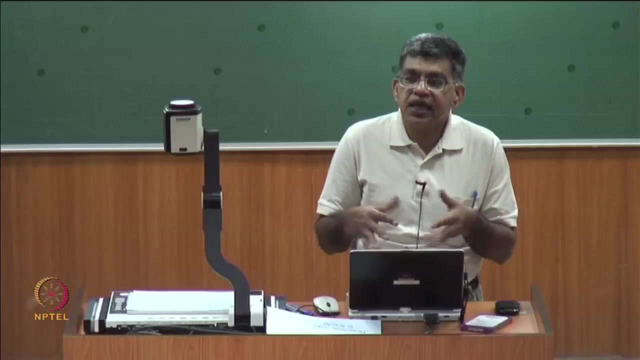 course, in the particular case when this m is 0 means that you have a constant, and instead of writing it as f with this purple parenthesis, very often we will simply write it as f. So that is our syntax of terms, and I have given them a separate color because they 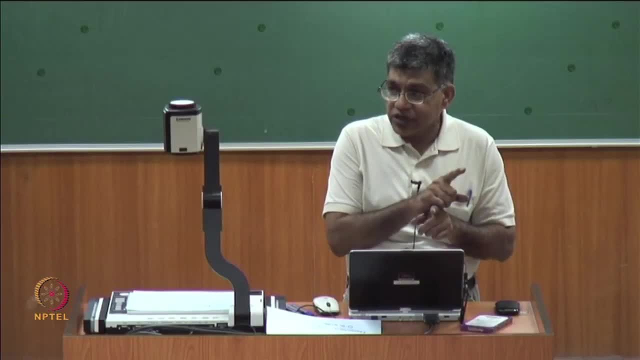 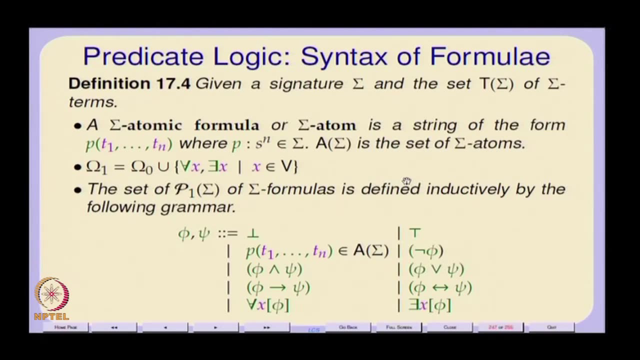 essentially specify your mathematical theory, except for the relations that are there in the theory for which we are going to have predicates. So, given a language of terms, already sigma terms, then you also have a collection of predicate symbols, So we will use p, q, r, etcetera for essentially for atomic predicate symbols. but now our predicate. 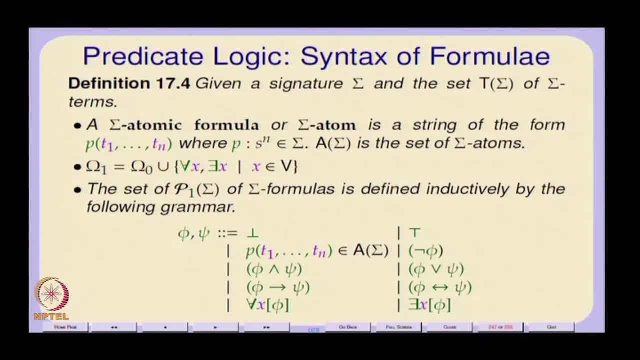 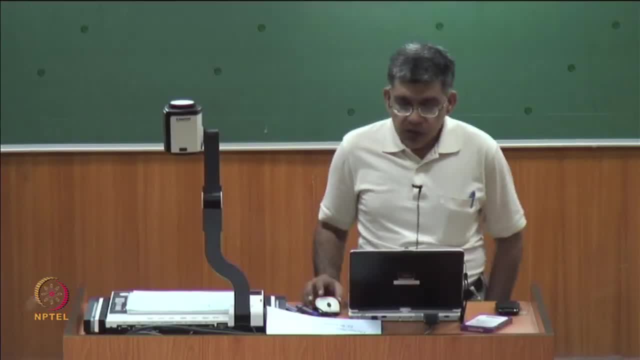 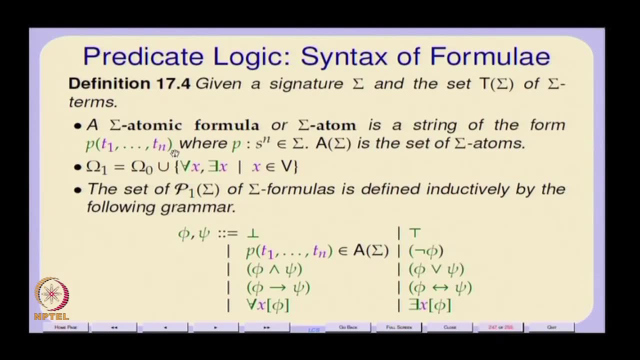 symbols are essentially propositional functions, So they take, they have places, empty places to be filled up. So an atomic proposition itself means that it will have, let us say, n variables, x, 1 to x, n, So it will have a propositional form in which these place holders can be replaced. 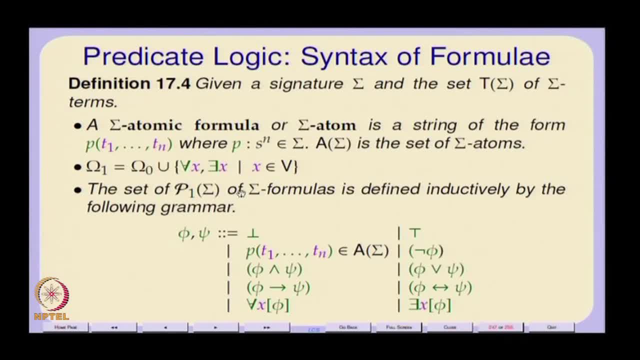 by terms t 1 to t n, and then we will have all the propositional connectives. after all, we cannot- I mean you are going to consider compound propositional forms too, So we will have all the propositional connectives that we had. I am now calling that set omega naught. 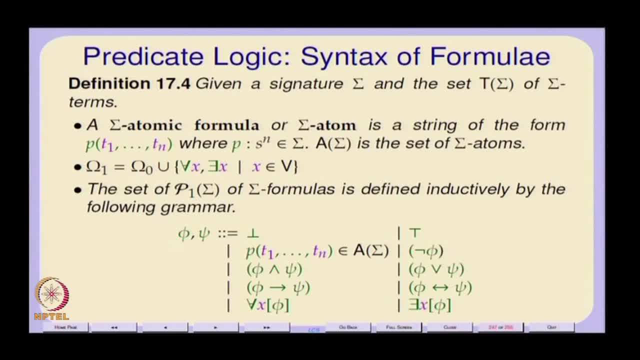 to signify that it is the there, all the propositional connectives like not, and and and or, and conditional and by conditional. And then, in addition, we have these two operators called the quantifiers. if you have an infinite collection of variables, v, you obviously have an infinite. 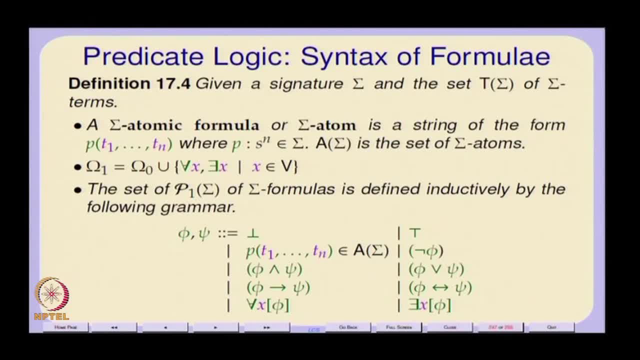 number of operators, One for each variable, one this is for all, one for all for each variable, and one there exist for each variable. So we have this, this is our signature, this is our collection of operators, and we will use phi and psi as usual, as typical members of the set of formulas. 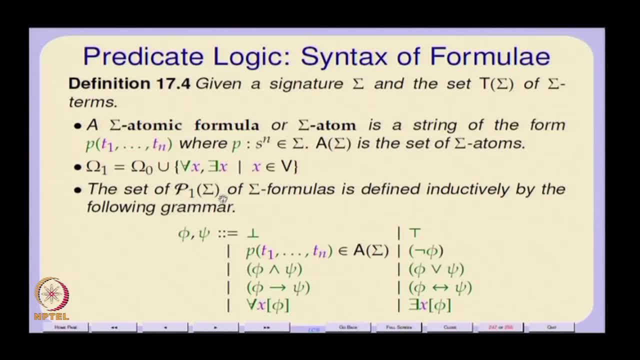 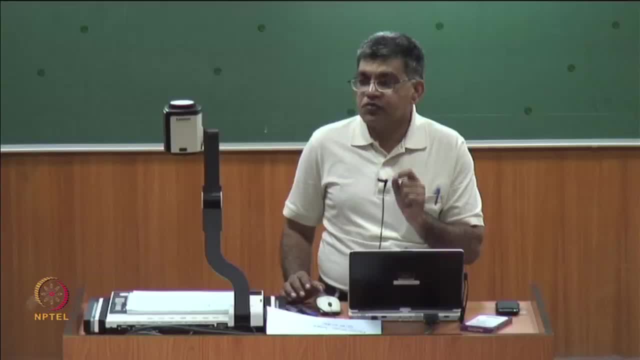 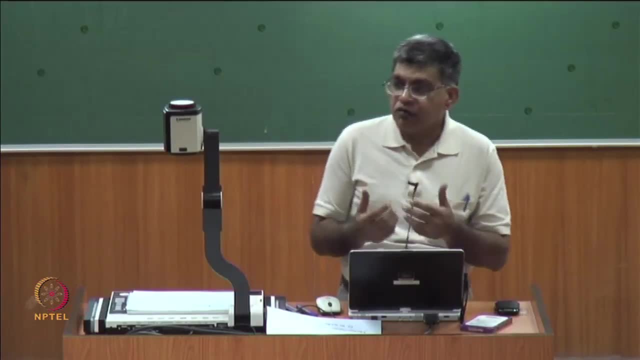 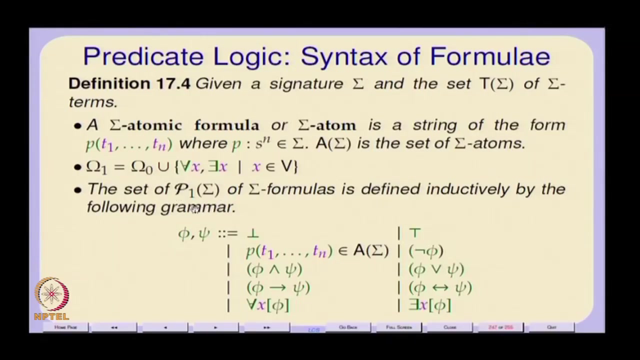 Now and the language now? I am calling it p 1 of sigma, propositional logic. I just call it p naught now, since it is parameterize And it is meant to describe some particular sigma algebra. we parameterize on sigma, so p 1 is a first order language For describing 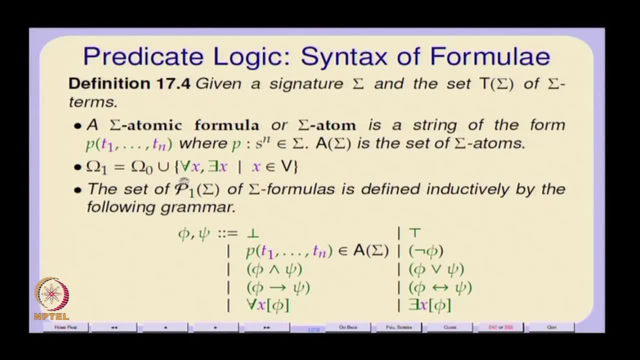 these for describing essentially the properties of a sigma algebra. So these sigma formulas are defined inductively this way, and here is my peculiarity, that is, that I like to specify the scope of variables, of a quantified variable, and I like to delimit them by square brackets. So otherwise I personally have had a lot of trouble just 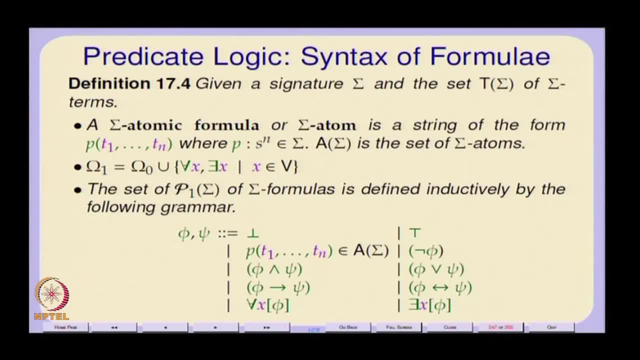 remembering precedences of operators and trying to figure out quantified formulae in text books. I find it is really painful. So instead, if you have a clear delimitation of scope, like we have in programming languages, it greatly simplifies matters. So, for example, now I do not need to talk about the precedence. 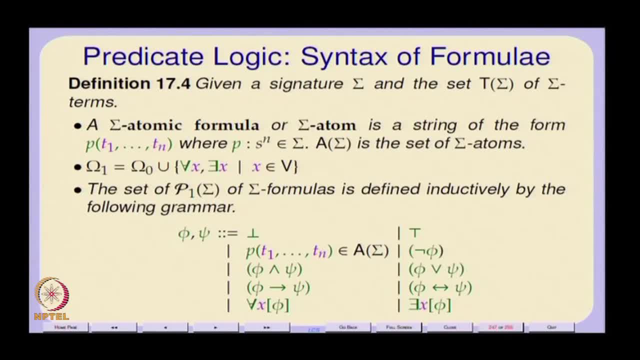 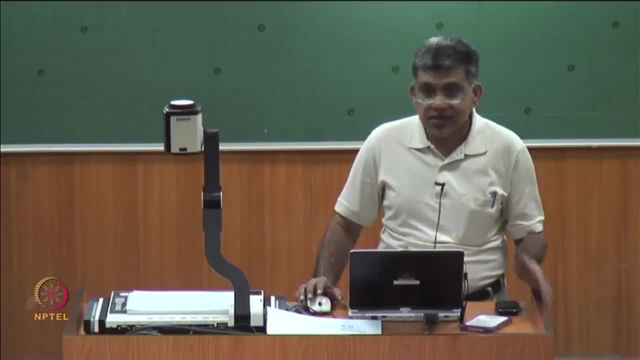 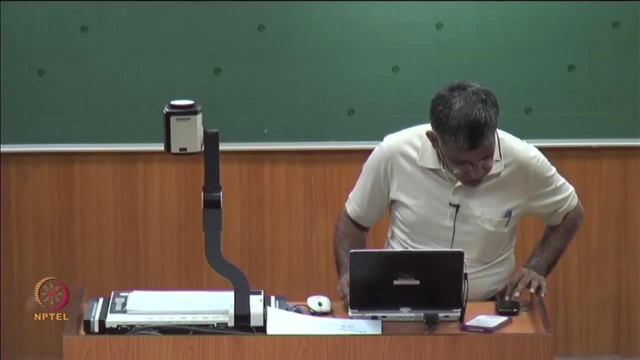 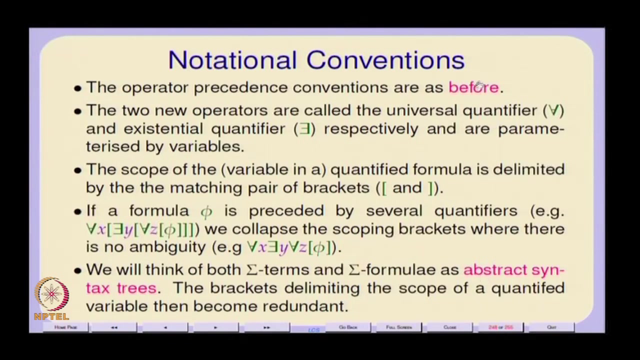 of operators in this case. So, and what is the extent of the scope is something that is clearly delimited by the brackets, though that is an extra piece of syntax. So the operator precedence conventions are as before. For these new operators, there are: 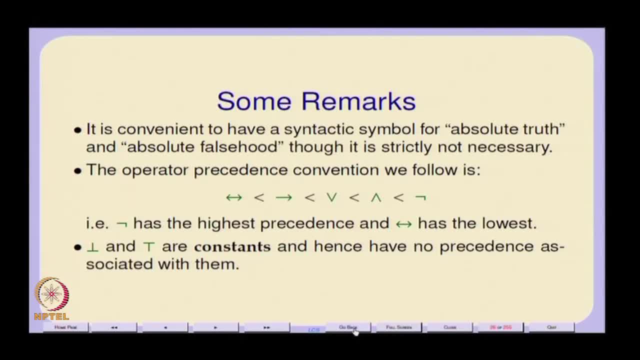 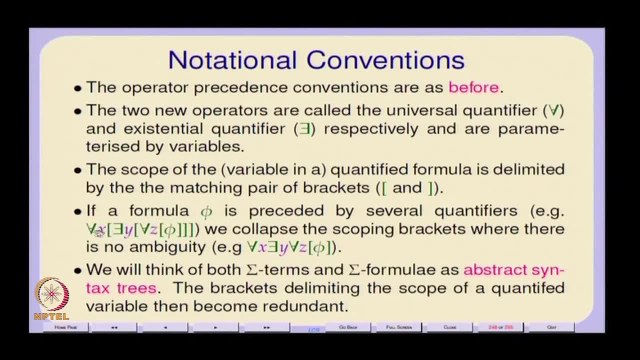 no particular new precedences, because any way, the square bracket should take care of it. However, what I am also going to do is that I mean I am going to have a shortcut. I mean, having too many brackets is also a terrible pain. So when you have a formula phi preceded by several quantifiers in sequence, with no other, 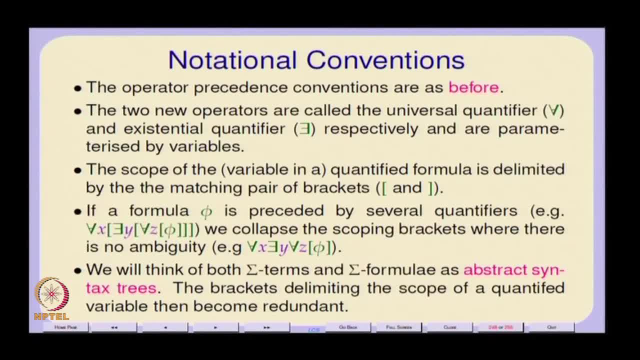 propositional or other connectives occurring in between. So if you just have a sequence of quantifiers, then I will just use a single pair of brackets to So instead of here, look at this: for all x, there exist. y. for all z, phi, which has three pairs of square brackets. 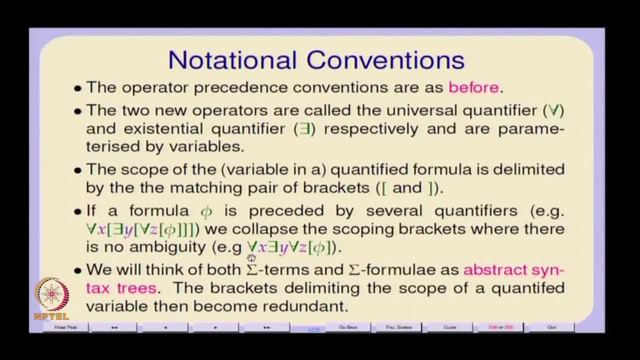 to specify the scope, But it is simpler to just specify it. as for all x, there exist y with a single pair of brackets around the phi. So this essentially tells you the scope. I mean it does not. you do not lose any information and it is simpler to write. So that is what. 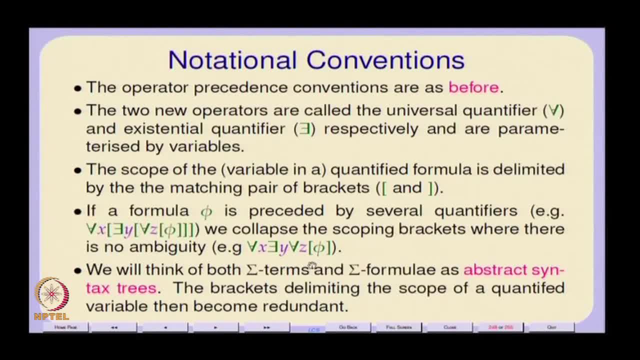 we will do So and of course, as before, we are not really interested in, like most logic books in these strings and distinguishing between these strings. we are interested only in the abstract syntax trees. This formula, any formula is, gives you an abstract syntax tree. So here is some here. 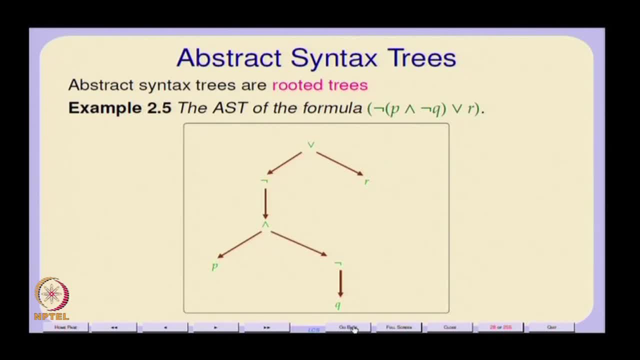 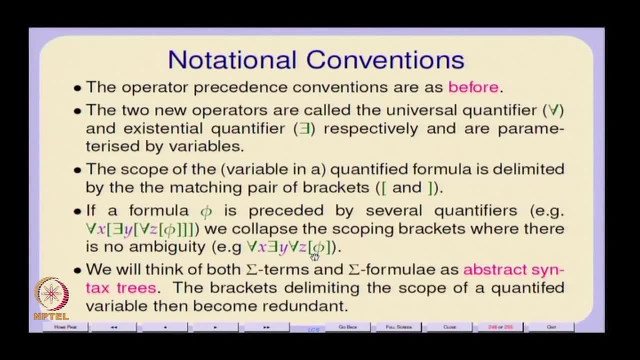 are some. this was a propositional formula, the an abstract syntax tree. And in an abstract syntax tree even the scoping brackets become redundant. I mean, you do not need them because scope also follows the tree structure. So it is actually So. we will think of them. 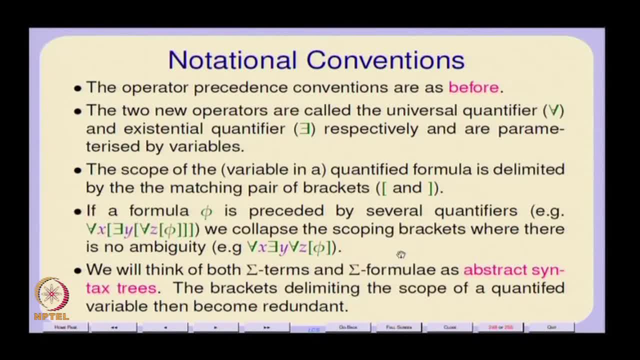 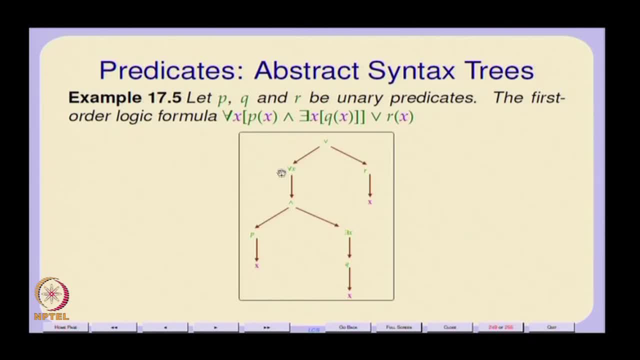 only as abstract syntax trees. So here I do not know where you can see all the operators here. I think it is the lettering is too small, But here is the formula and this is like for all: x, p, x, and there exists. 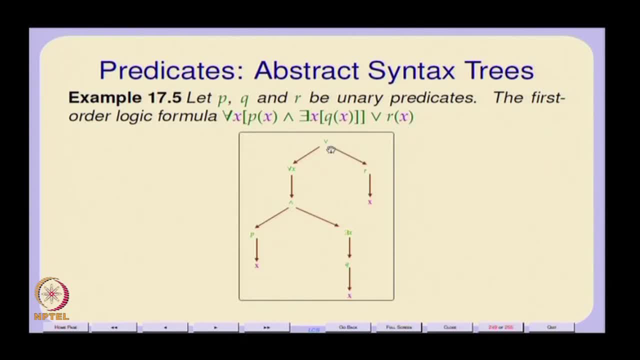 x, q, x or r, x. this is the abstract syntax tree. For that the root operator is this or, and then r is So the r abstract syntax tree- text tree of course- starts with predicate symbols and then becomes terms. the terms are: 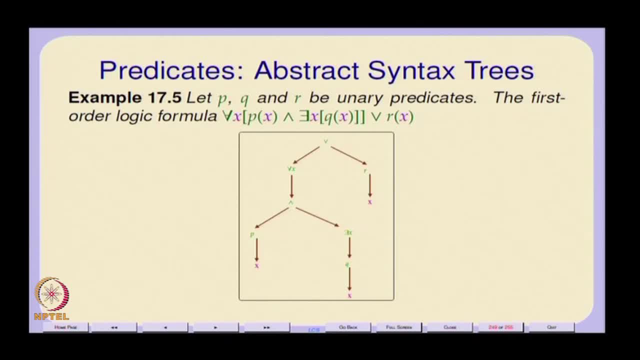 also. I mean they are also abstract syntax trees on the predicate symbols. So for example I can have: so here there exists q, x, and here is an, and here is the this and p of x and this or is, and then there is an universal quantifier for all x here, and this is the abstract. 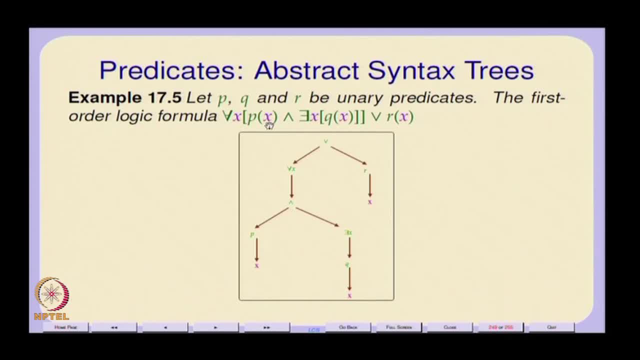 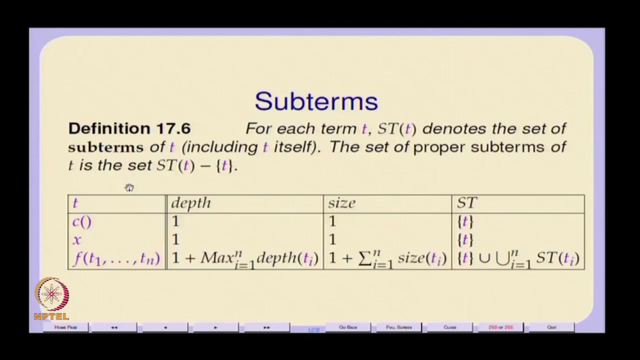 syntax tree of this formula. If, instead of x, I had some complicated term, then that would have come here, for example. So we have green labeled nodes which gradually go into violet labeled nodes, basically, you know. So abstract syntax trees would look something like that: 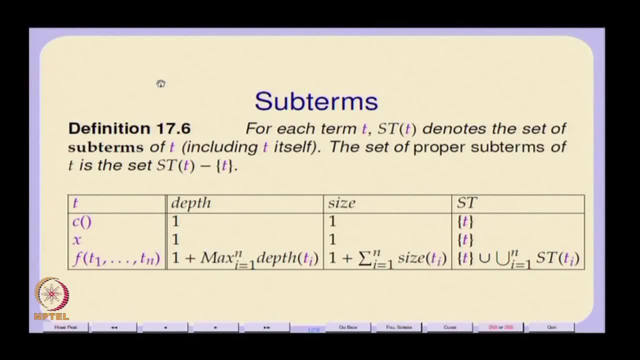 there is a far more amount of technical stuff related to the syntax That we need to worry about, because now we have got the notion of, now we have got notions like free variables and bound variables, notions like sub terms and sub formulas. So we have 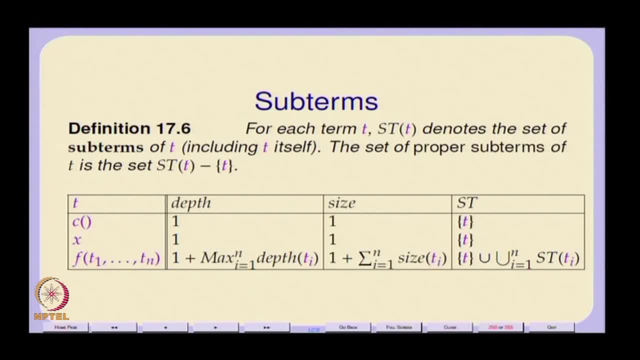 a hierarchy. now, clearly we have a two level hierarchy. there is a hierarchy of the language of terms and above it there is the hierarchy of the language of predicates, and you cannot mix the two. Your all your abstract syntax. trees should, at the root, look green. 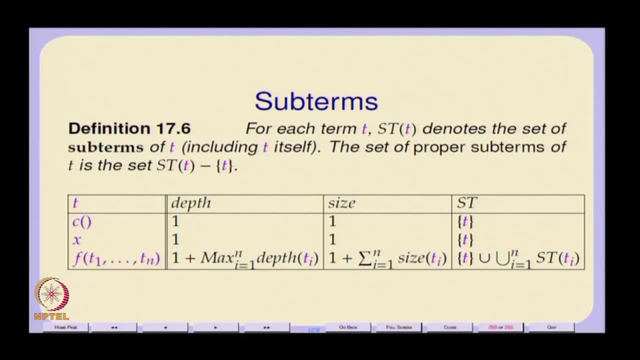 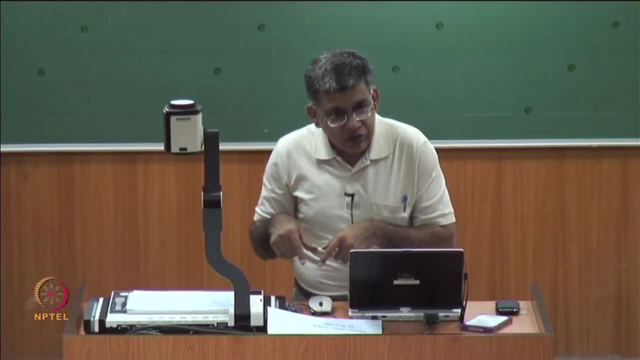 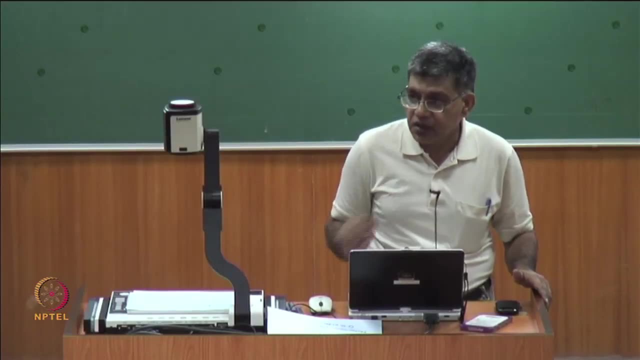 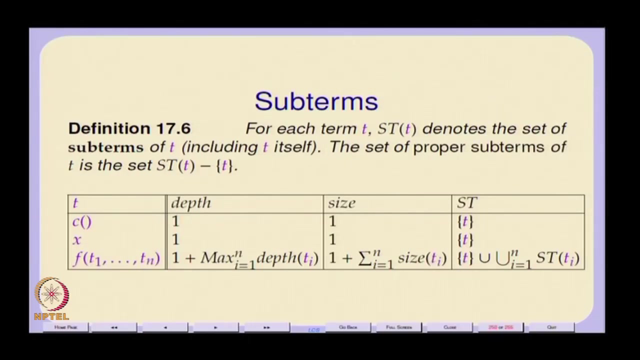 They should either be completely purple if they are terms, or they should start from somewhere green and then start becoming purple and from within that purple they cannot change to green, for example. that is So you have a hierarchy of. we have a two level hierarchy of terms and predicates, So naturally it brings in, so there is a notion of sub terms. 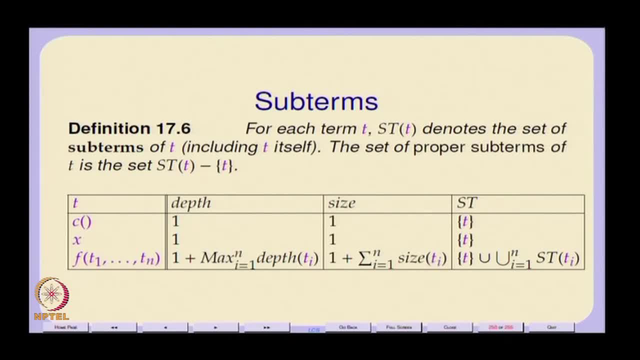 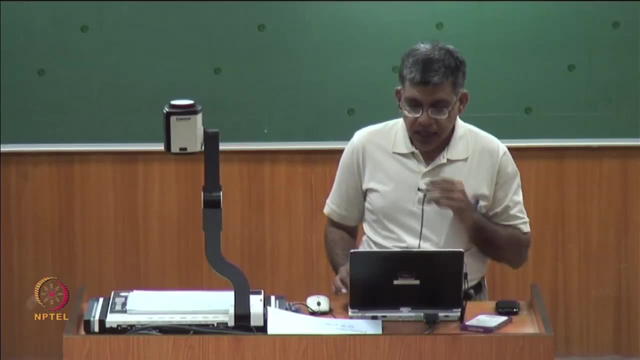 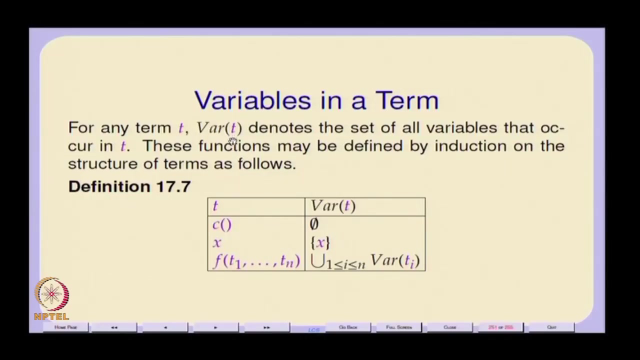 for a term, and these are certain measures that will be useful for performing induction, like depth, the size of a term and so on and so forth, Which can be defined by induction on the structure of the terms and similarly. but the other complication which quantification brings us is the notion of a binding and scope and 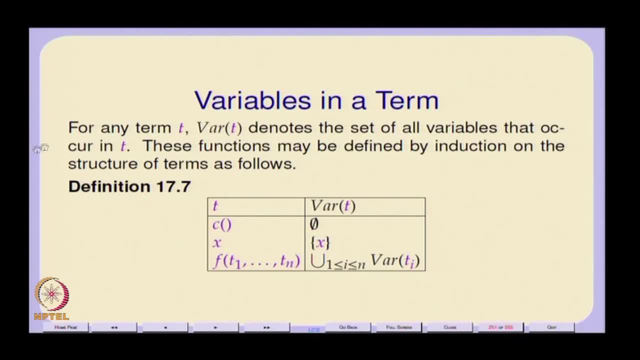 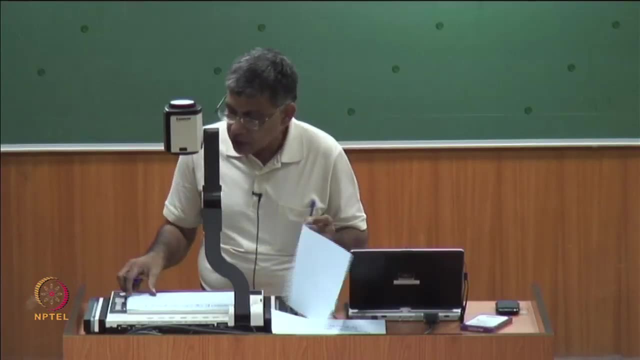 the notion of, therefore, free and bound variables. So we will, in any term. of course, there is something, there is another simplification which we have done: remember that our language of terms did not have a problem of free or bound variables, Whereas, strictly speaking, 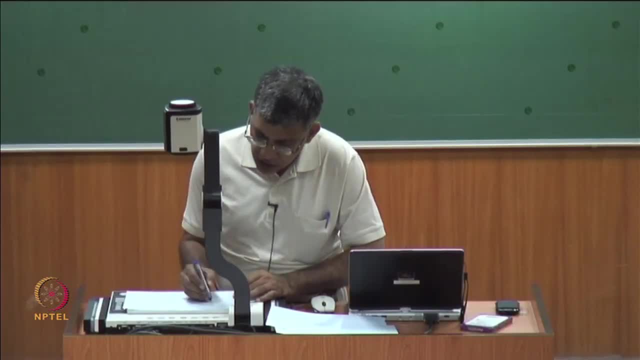 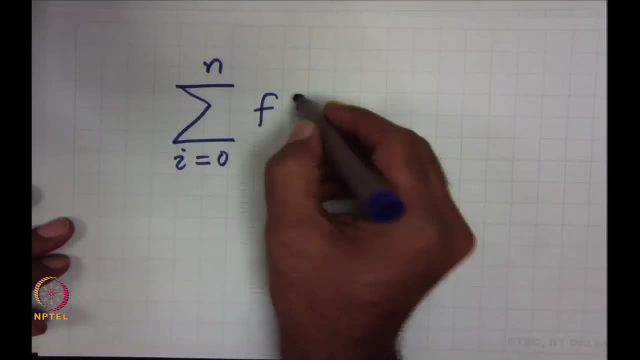 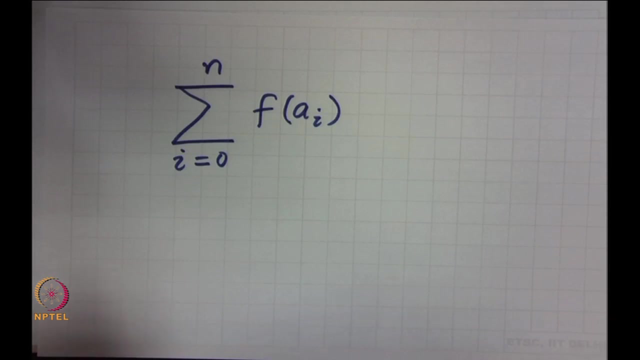 if you have, if you have, even if you have even simple things like this, if you have simple things like this And notion of free and bound, variable's actually have to come up, because even in the language of terms- but we are simplifying life, I mean. 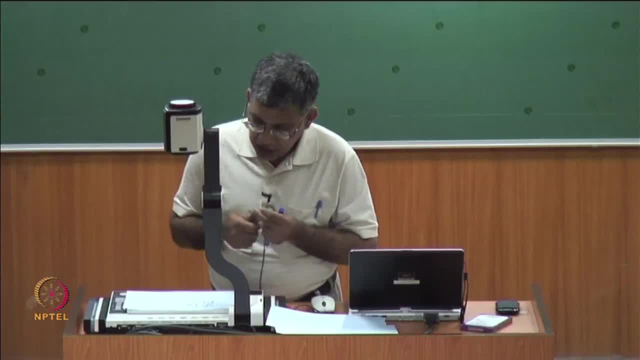 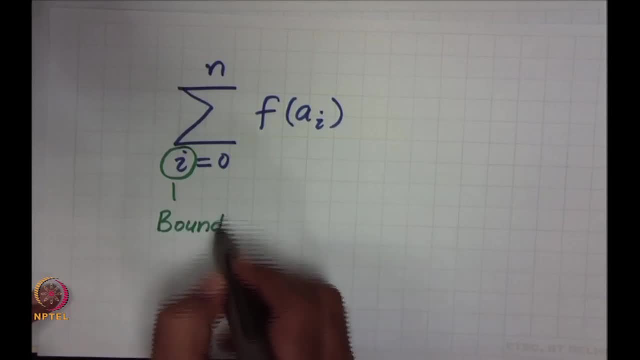 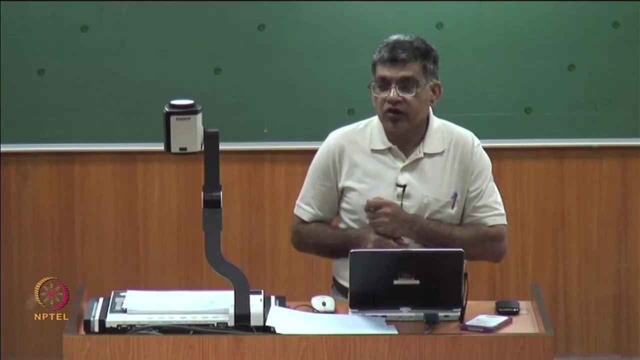 for example, this is a, this is a bound variable, ah, whereas this is free. So, however, we are not our signature. we have specified it in such way that there are no And therefore there is no concept of a bound variable in terms. So that is a simplification. 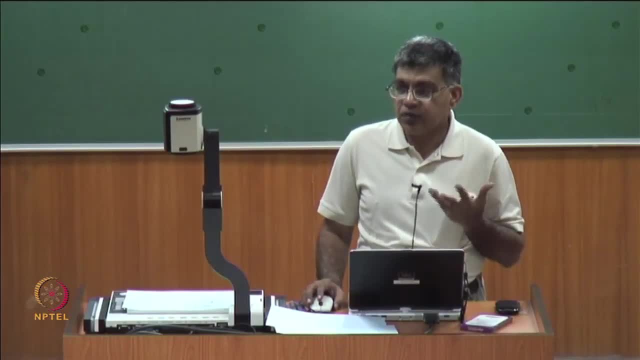 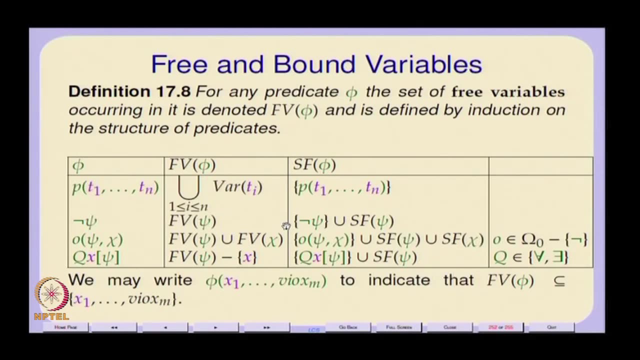 that we have done, But so we will just look at the variables in a term, and that can be defined by induction on the structure of the terms. You need the variables in a term in order to be able to define free and bound variables on predicates, Because your terms form the underlying sub trees of your predicates. So 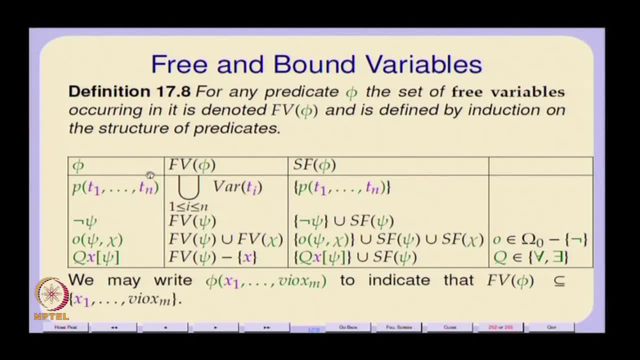 we will define for any predicate phi, we will define f v of phi to be the set of all free variables And, of course, given an atomic predicate p of t 1 to t n, where t 1 to t n are terms, you just take the union of all the variables. 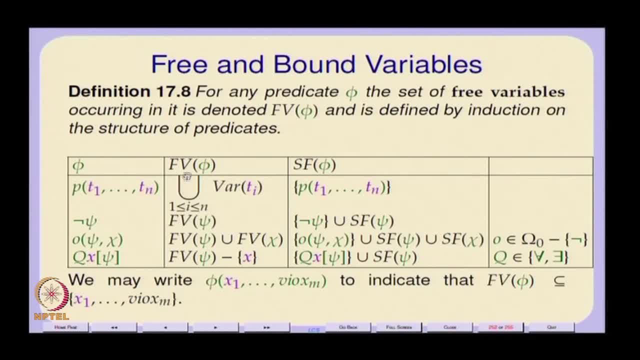 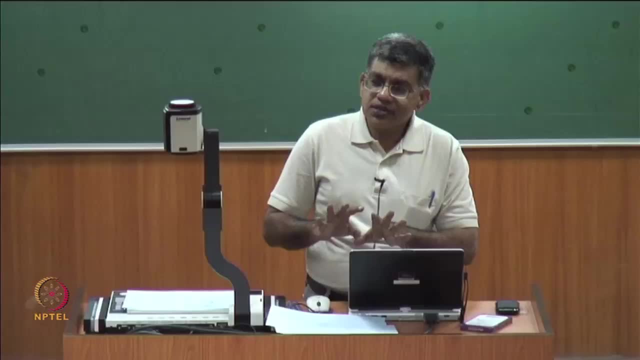 in that, In each, in all the terms, and that is the set of free variables. And we also sometimes require the notion of a sub formula. But the notion of a sub formula is actually quite trivial. the notion of a sub formula is just that of a sub tree of the abstract syntax. 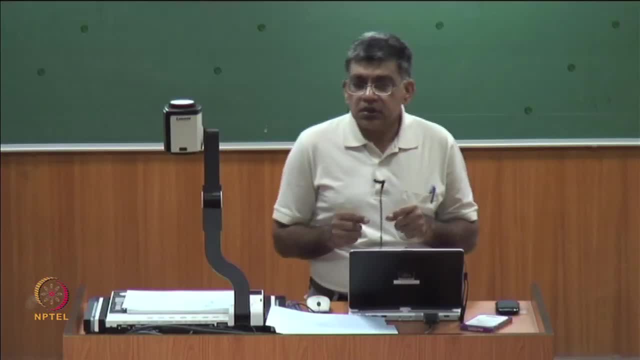 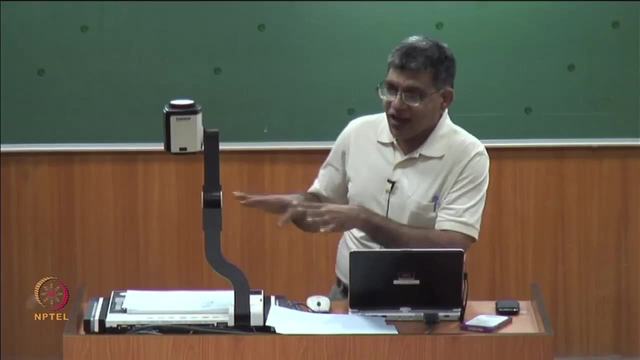 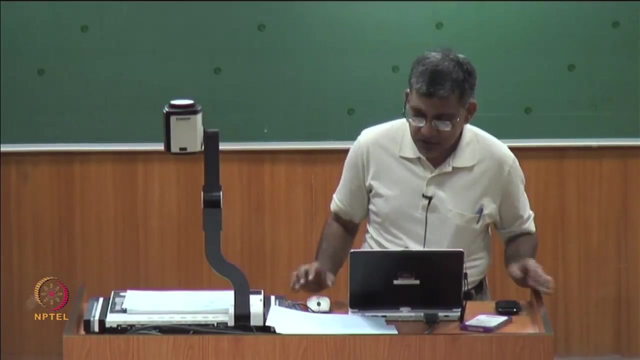 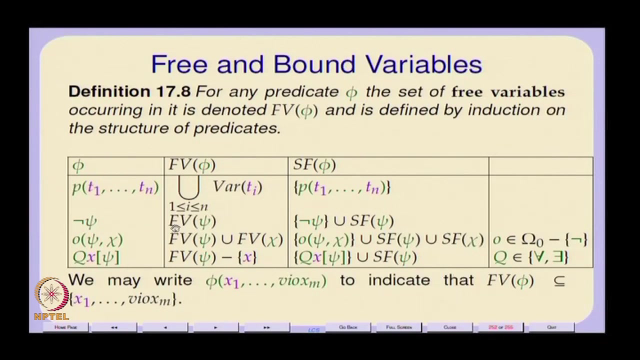 tree, Except that you should not look at sub trees of terms as sub formulas. I mean, Pablo, Un lado The violet, the sub formulas should still have something green at the top. I mean they cannot just be violet. So, and in the case of not formula, of the form, not psi, you just have free variables. 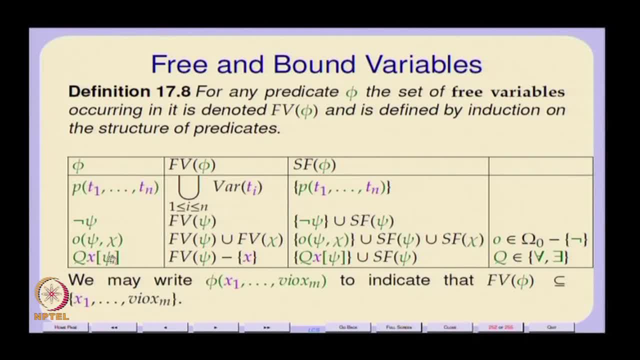 of psi And the set of sub formulas is just this For any of the propositional connectives, except not. you just take the union of the free variables of the two components. we have all of them: 이 좀, operators, and similarly you also define your sub formulas as unions like this: 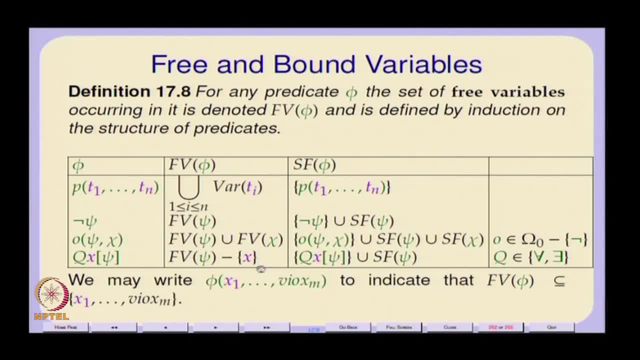 And for any of the quantifiers, you remove the quantified variable from the set of free variables of the body of the quantified formula. So this, whatever is within the square bracket, within the scoping bracket, is called the body of the quantified formula and x no. 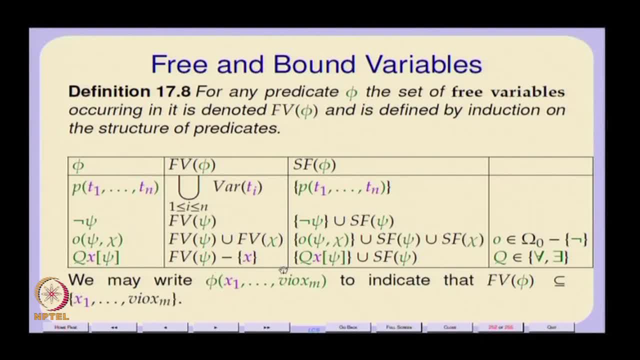 longer remains in that because x is a boundary. So I am sorry this should have been changed to: I think there is. I forgot to put a backslash. So this is x 1 to x m, all in violet color actually.